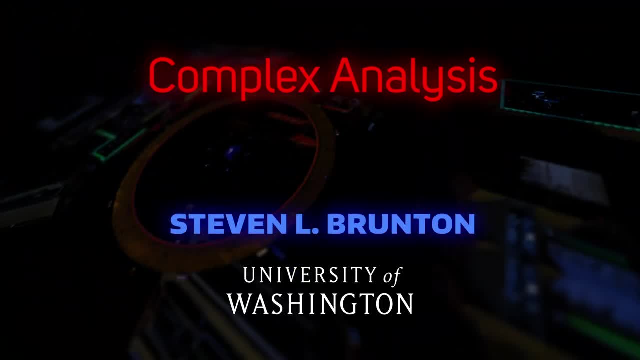 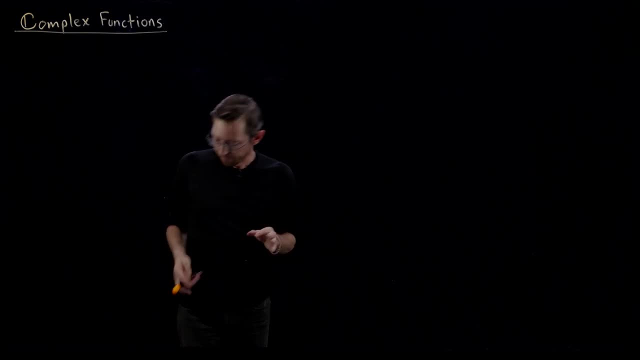 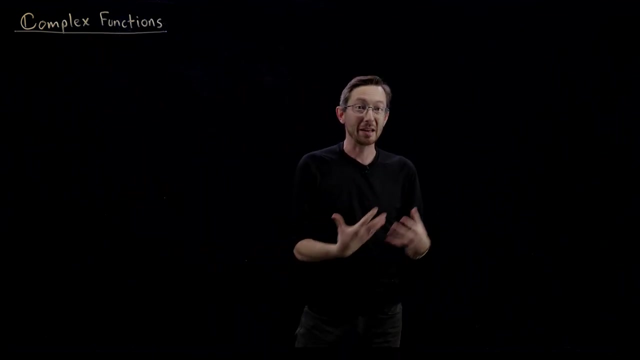 Welcome back everybody. Okay, so it's been one week in the complex wilderness and today I am ready to tell you about one of my favorite properties of complex functions. So I'm going to define what it means for a function to be analytic, And analytic functions are essentially well-behaved. 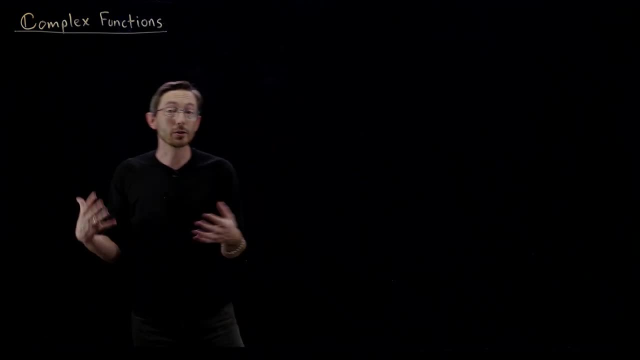 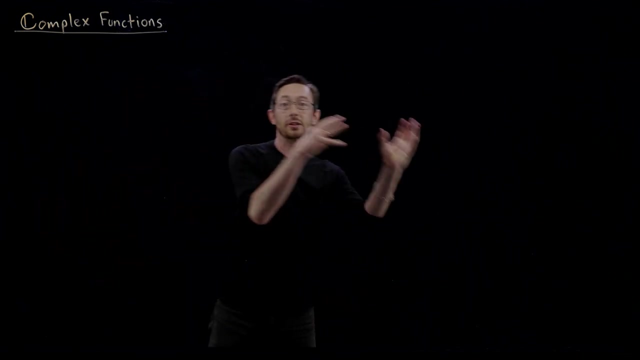 functions that we can do calculus on. Okay, so we're used to doing taking derivatives and doing integrals for real valued functions and we would like for all of that to carry over to complex functions because, again, remember, these complex functions are going to be how we represent the 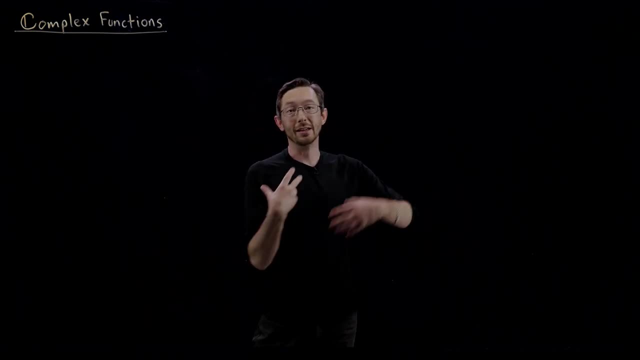 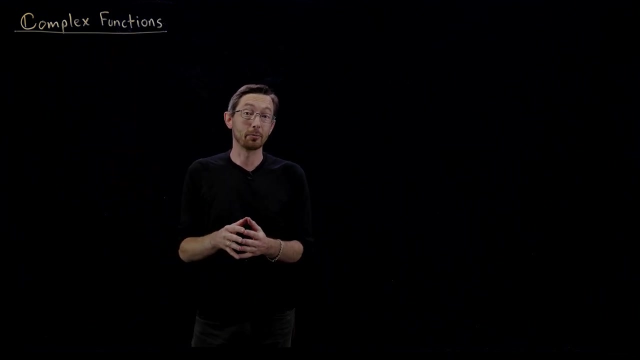 solutions of ordinary and partial differential equations. So we need to be able to take derivatives and integrals and do calculus. And some functions in the complex plane are actually pretty wild and poorly behaved and break our intuition of what it means to be able to do. 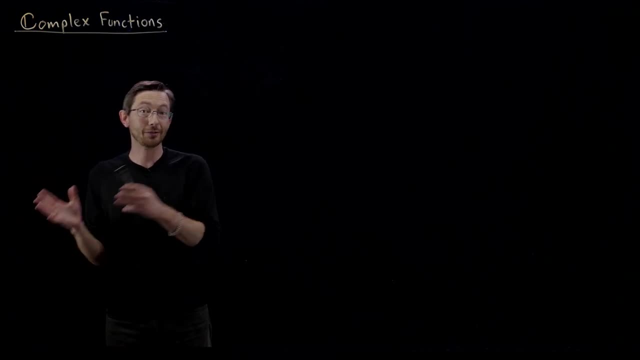 calculus, So some functions are better behaved than others, and the well-behaved functions that we can do calculus on are typically called analytic functions. Okay, so specifically, we're going to be talking about analytic functions. Okay, analytic functions- Very, very important. 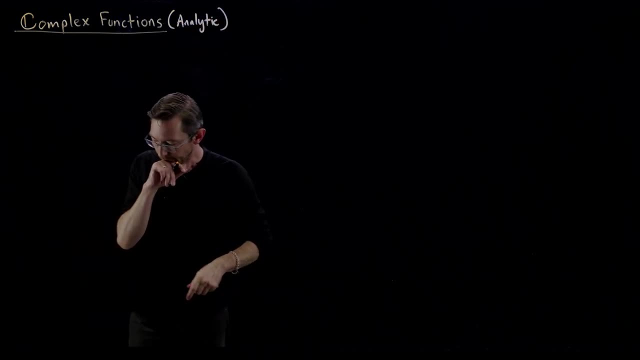 class especially for solving partial differential equations. So a function, and I'm going to define it, then I'm going to give you an example of a non-analytic function to show you how things get weird, and then I'm going to give you conditions to know if a function is or. 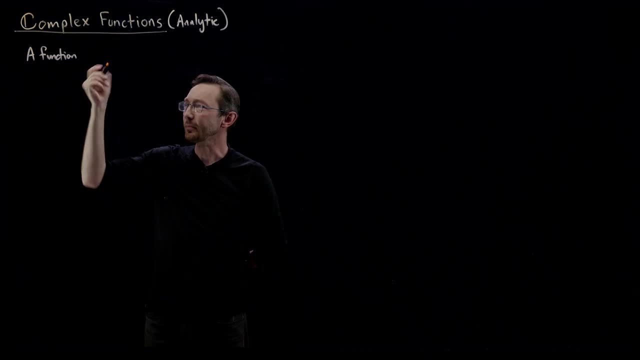 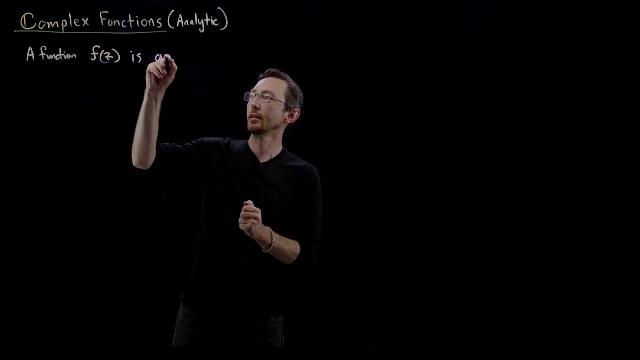 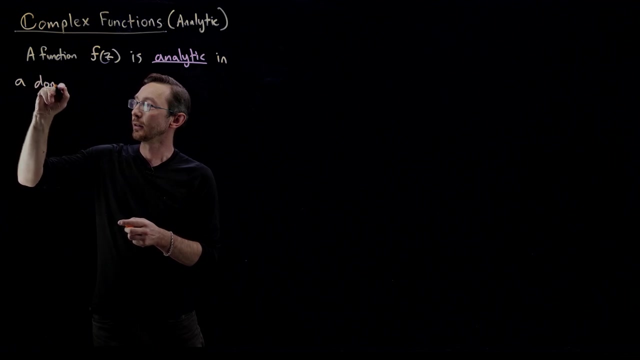 is not analytic. So a function, let's say f of z, is analytic- and I'm going to use red for this- is analytic And we typically say it's analytic in a certain region of the complex plane. so in a domain, a domain is just a region, it's math speak for some you know, set in the complex. 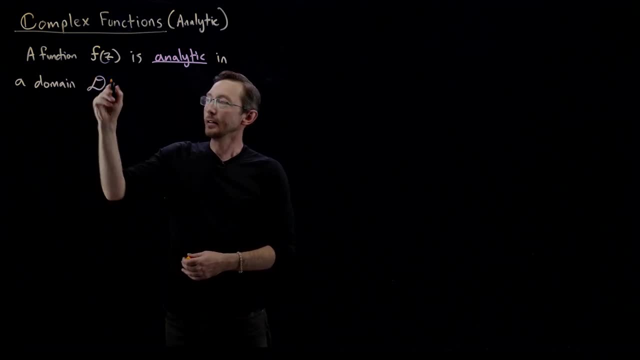 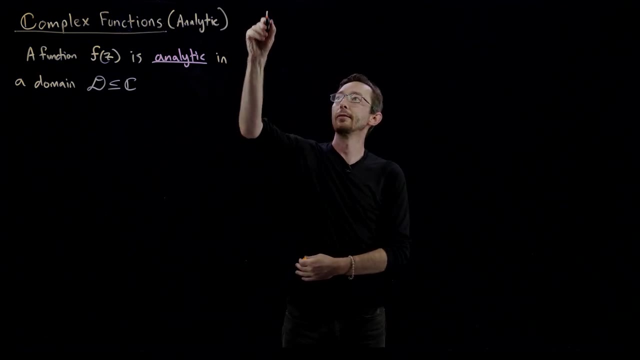 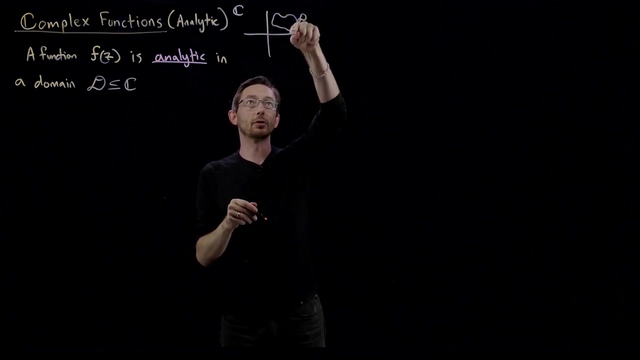 plane, some domain d in the complex plane. in the complex plane it could be equal to the complex plane, it could be the whole plane or it could be a little subset. So if I have my complex plane then my domain is just some, you know some little region where I'm talking about some subset. 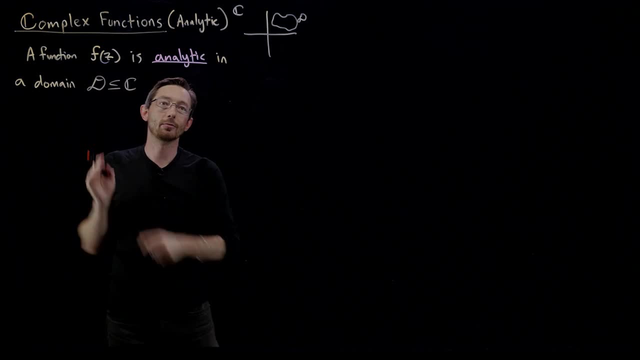 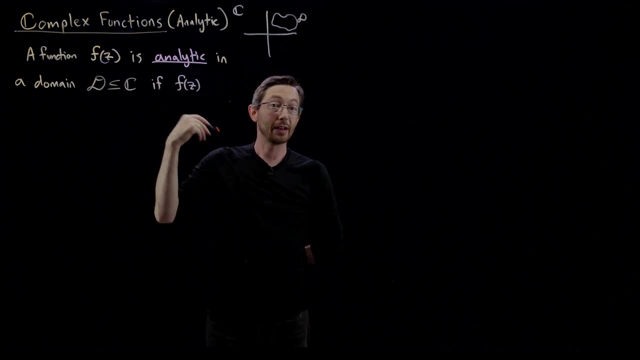 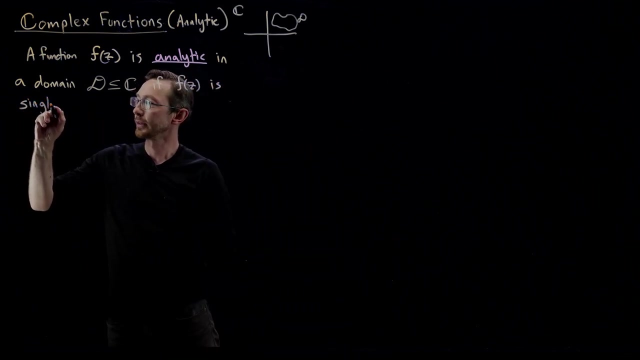 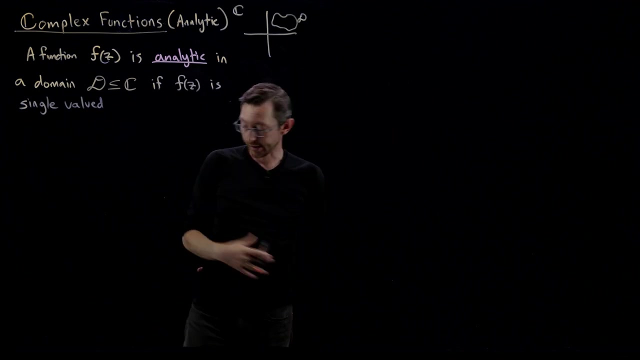 A function f of z is analytic in that domain. d, if f of z is single valued- remember the logarithm was infinitely valued. so if f of z is single valued, single valued, like the cosine and sine functions, are single valued. z squared is single valued. z to the one half is not single valued. 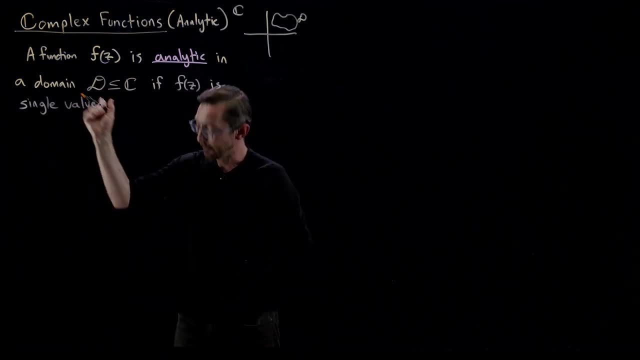 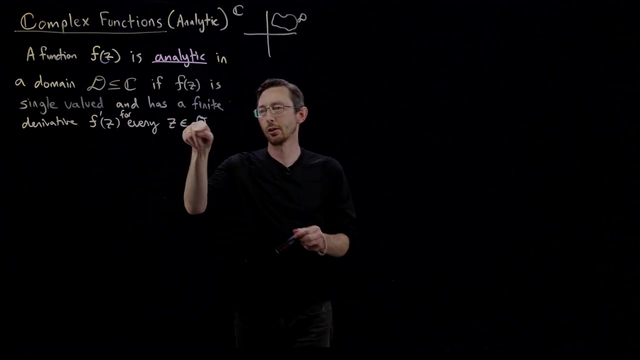 there's two solutions to z to the one half. there's two solutions to z to the one half if it's single value and has a finite derivative, derivative f of z, f, prime of z everywhere, or let's say, for every z in that domain, d. Okay, this is just curly d. 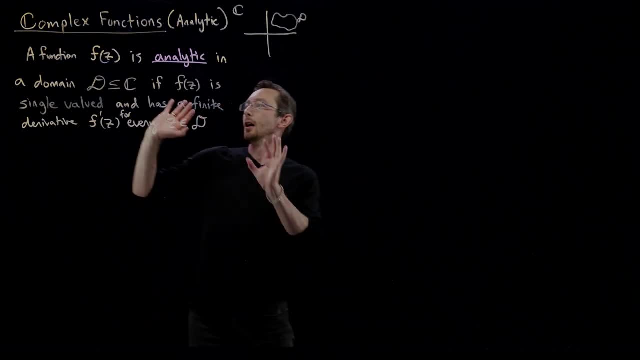 sorry it looks so squiggly, that's my fancy pants. d. Okay, so this is just math words and these are the conditions. I'm going to show you that. these are the conditions for that function f for it to be well behaved enough for us to do calculus on. We can take derivatives. 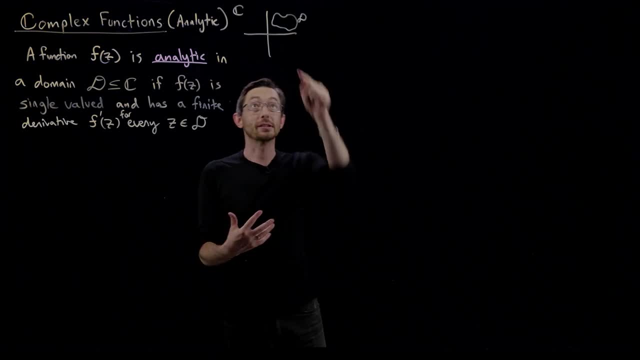 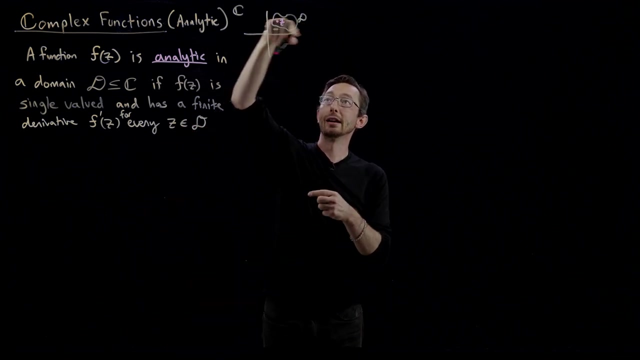 and they mean something intuitive to us. we can do integrals in that domain d, and there are special nice properties if f is single valued and there exists a finite derivative at all points in that domain. So we're talking about points z that are inside this domain. that's what's. 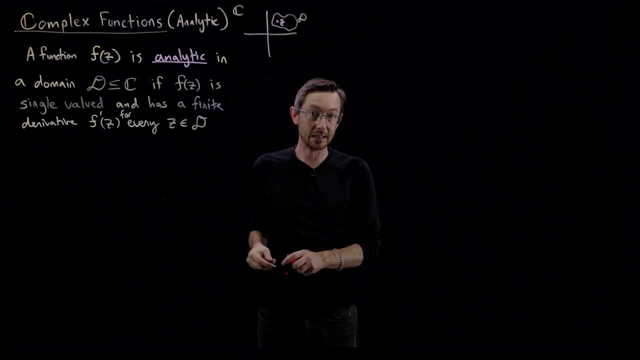 what this is. in math speak, z is an element of the set d, the domain d. Okay, so we already know about functions that are not single valued. z to the one half has two values. z to the one third has three values. log of z has infinitely many values. so those are going to kind of 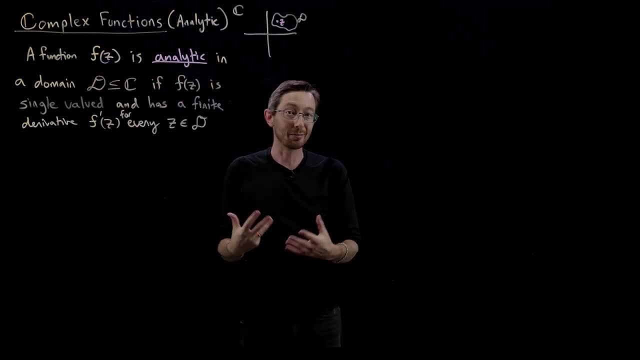 break immediately. this definition of analytic and calculus is going to be weird, or at least slightly different. on those functions. Functions like z squared are going to be fine. they're going to have to be single valued and it has to have a finite derivative for every z in the 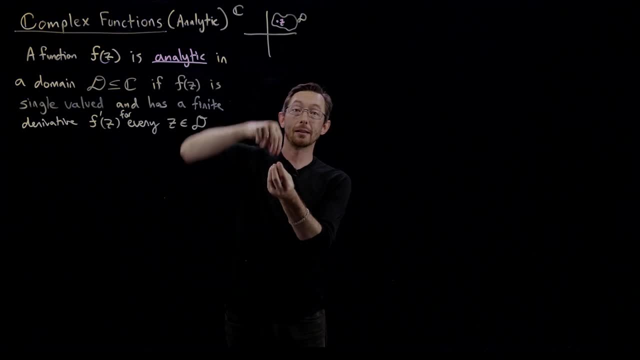 domain. So, specifically, the derivative can't be infinite. it can't be. like you know, the function one over z is going to blow up at z equals zero. it has an infinite derivative and the derivative is going to have to be the same, no matter what path I take that derivative in. Okay, so I'll. 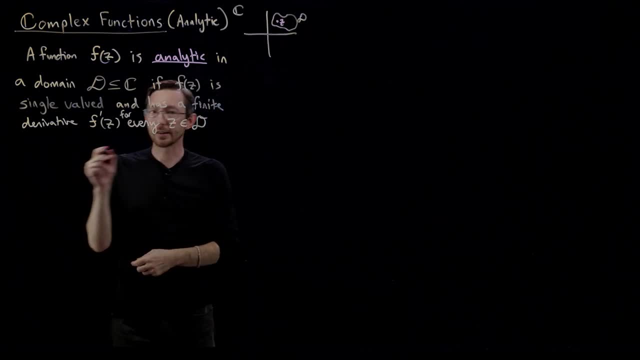 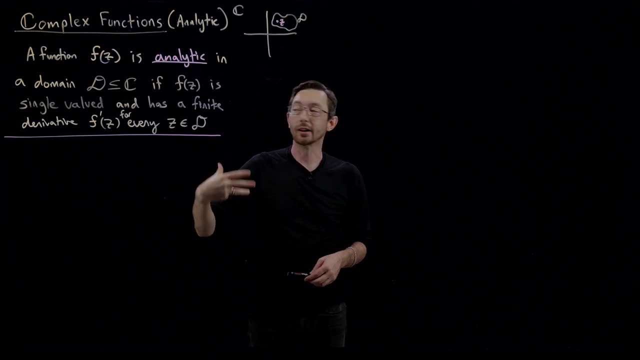 tell you what that means in a minute. Good, So this is a kind of a definition, and what I want to do now is I want to give you an example of a non-analytic function to show you the kinds of weird things that can happen in the complex plane. So a non-analytic- 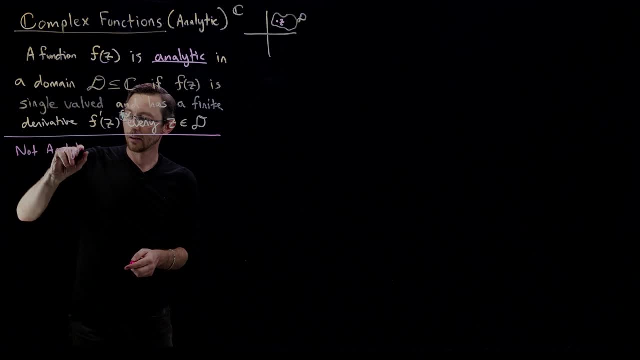 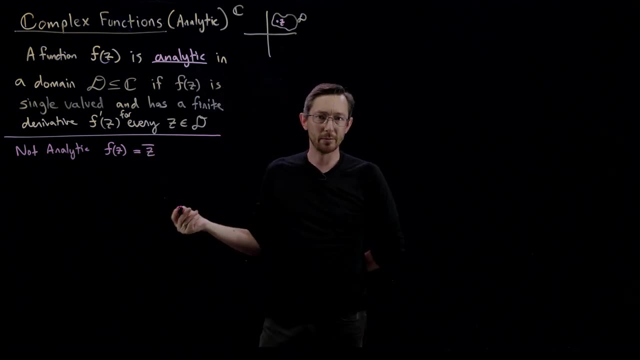 function, not analytic function, would be: f of z equals the complex conjugate of z, which we call z bar, which is equal to the real part minus i times the imaginary part. So, instead of x plus i, y, which is z, the complex conjugate of z is equal to the real part minus i times the imaginary part. 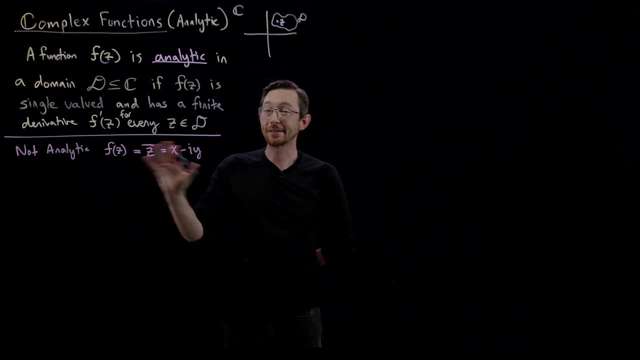 The complex conjugate is x minus i, y, and I claim that this function is not analytic, We are not going to be able to do normal calculus and in fact, what I'm going to show you is that the derivative doesn't exist uniquely. It doesn't have kind of a unique, well-defined derivative. 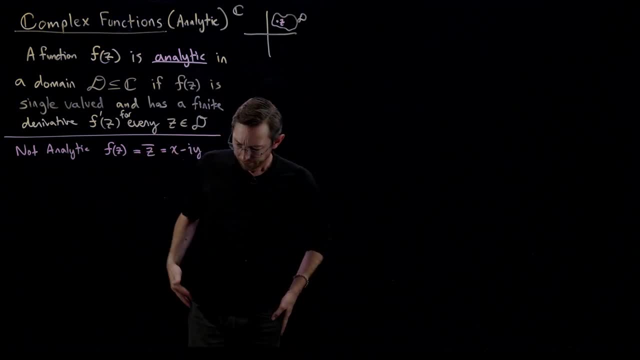 of this function. It's a weird function, okay. So let's see, I think what I want to actually show you is we're just going to compute the derivative and I'm going to show you that weird things happen. So we're going to take df dz. 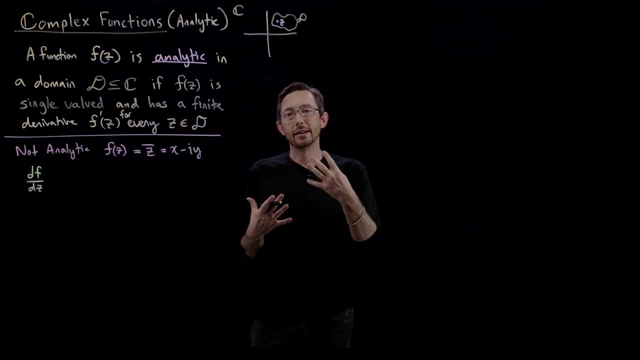 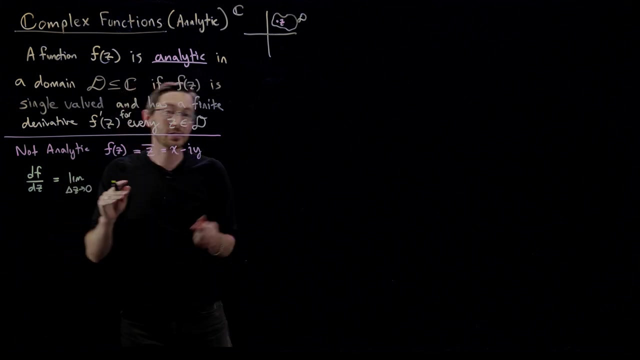 and remember that the definition of a derivative is essentially this kind of infinitesimal rate of change of f as I vary z. So this would be kind of the limit as delta z goes to zero. so my infinitesimal delta z goes to zero of f of z plus delta z minus f of z divided by delta z. okay, 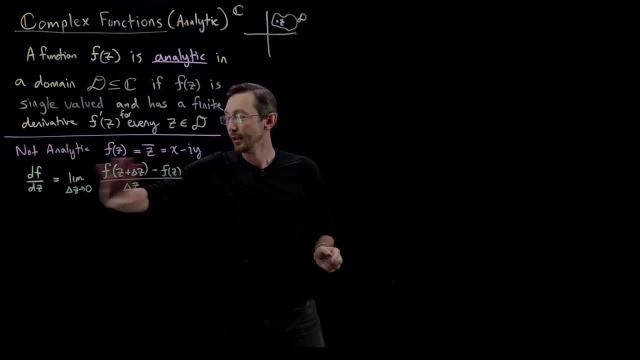 This is just standard. you know, freshman calculus kind of this is how we always have defined the derivative. This is how we're going to define the derivative in the complex plane too. totally legit, And so you know, that's essentially the limit of, let's say, this is. 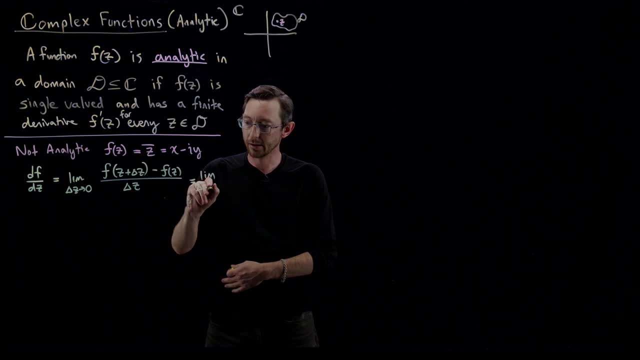 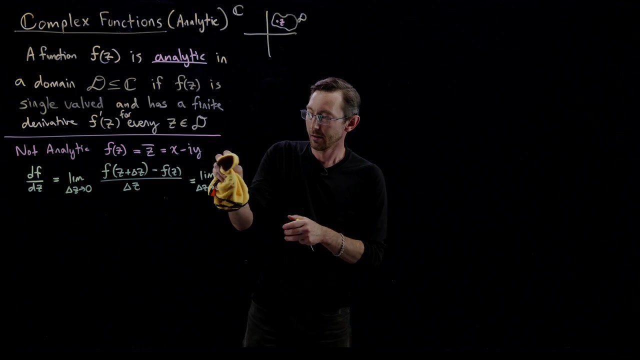 the limit as delta z goes to zero of z bar over delta z. That's just. you know, f of z is equal to f of z plus delta z minus f of z over delta z. I'm sorry, I should have said. 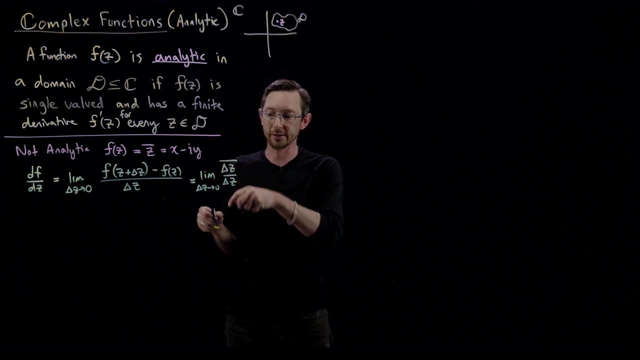 this is delta z bar, delta z bar over delta z. You can convince yourself that if you plug in z plus delta z to z bar and z to z bar and subtract them, what you're going to get left is a delta z bar, a complex conjugate of delta z, And this equals the limit, as 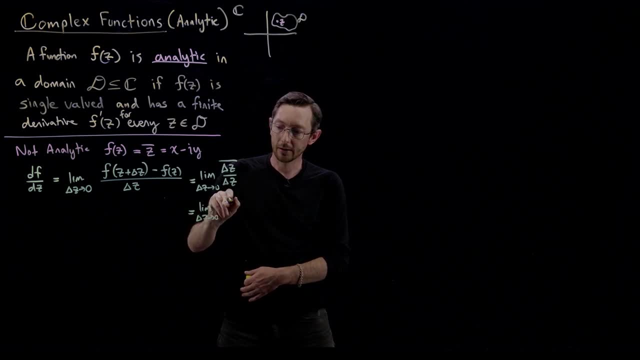 delta z goes to zero of delta x minus delta yi over delta x plus delta yi. Good, So the derivative df dz is the infinitesimal rate of change of f when I vary delta z. And if you literally plug in z plus delta z and z into this complex conjugate function f and cancel them out, 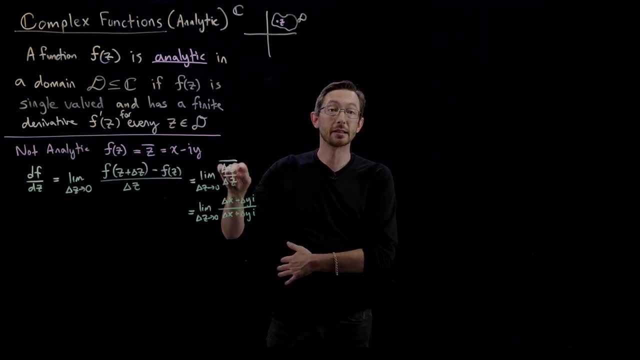 pause the video and do that. you'll see that the top is going to be delta z bar and the bottom is just delta z and we're going to take the limit, as delta z goes to zero And it's equal to this quantity here. okay, where you know, delta x is how much I vary in the. 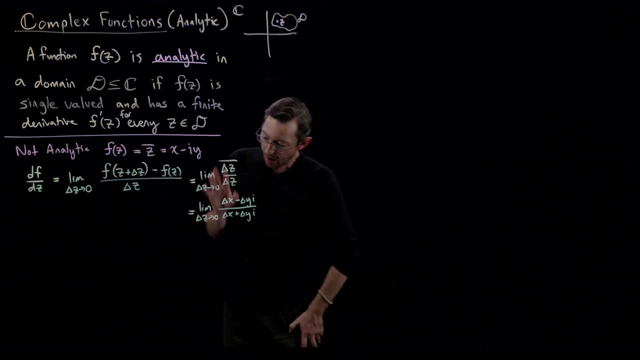 x direction. delta y is how much I vary in the y direction. But this is where it gets really weird is that this derivative is totally different if I take delta z- infinitesimal- and approach infinitesimal changes in the y or the imaginary direction. So that's what I'm. 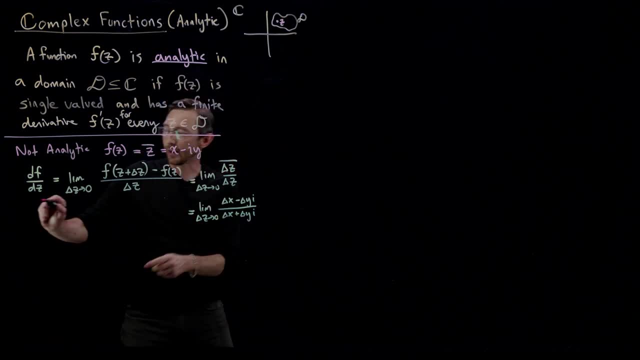 going to show you here. Okay so, and let me just define, so we're going to you know, let delta z equal delta x plus i delta y. That's what we define. delta z here, delta x plus i delta y And delta z bar equals delta x minus i delta y. That's what we have on the numerator. okay. 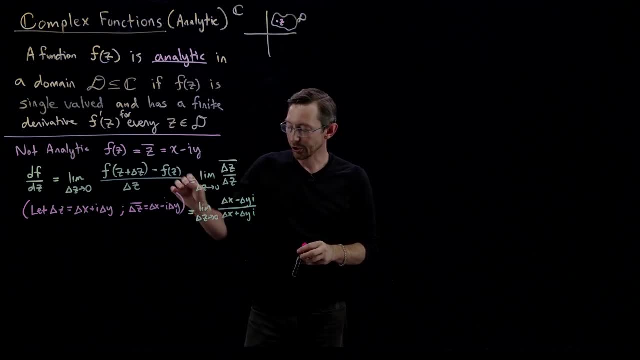 So now what we're going to do is we're going to look at this function as we approach this derivative. as we take this delta z goes to zero in different directions, okay, And so essentially, this delta z, I could- I'm just going to draw a picture here. actually, I think 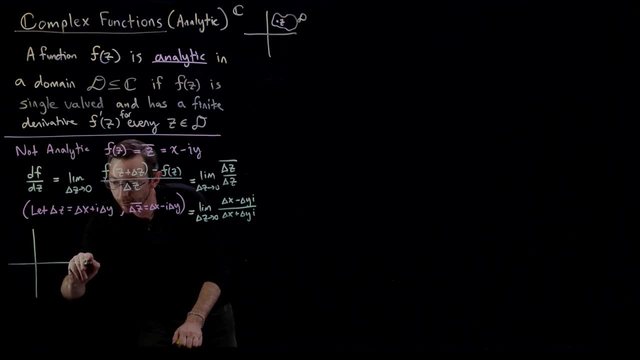 this is going to make it a lot clearer. So this is the real part, This is the imaginary part. Let's say that my point z is right here at the middle, And what I'm going to do is I'm going to look at case one. 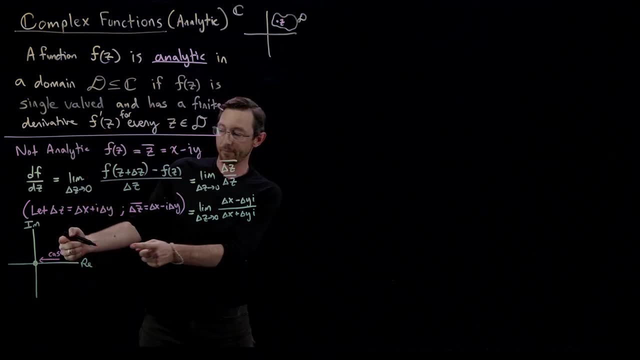 Where I take delta x goes to zero. So I'm going to start on the real axis and approach as delta x goes to zero. And then case two: I'm going to freeze the real part to zero And I'm going to take the limit as delta y goes to zero And for the derivative to make sense, those two limits. 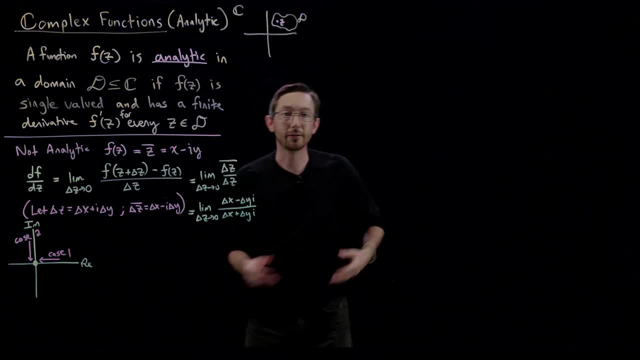 should be the same thing, okay. So, regardless of how I approach, delta c goes to zero, I'm going to this derivative should be the same thing, no matter what direction I approach, delta z equals zero. okay, And so if we write this out, so if we say you know, let's say approach, you know. 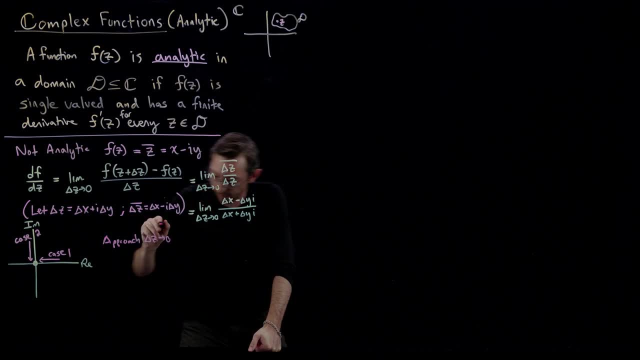 approach. delta z goes to zero from real axis. from the real axis, which means delta y starts out being zero, And then I take the limit, as delta x goes to zero, And then I take the limit, as delta x goes to zero. This is case one. Then that means the limit. this expression becomes limit as delta. 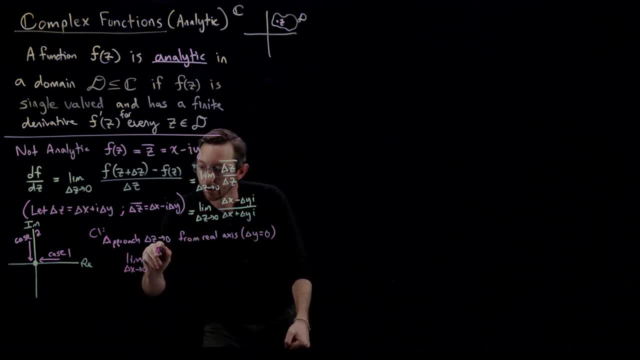 x goes to zero of delta x over delta x, That equals plus one plus one. okay, So the derivative of this function, if I you know, started with delta y zero and I take the limit as delta x goes to zero. I approach from this direction. in case one, my limit equals one. So this in case one, I'm 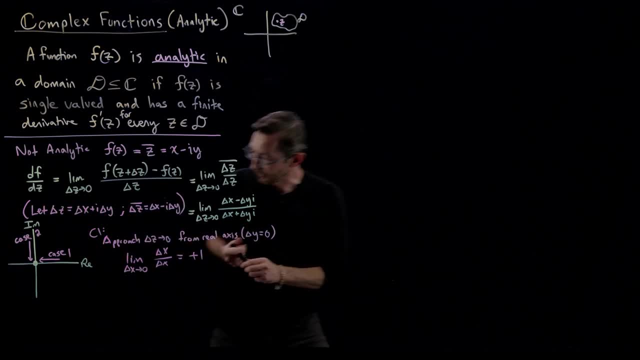 this directional derivative is equal to one. Let's look at case two. when I approach in the imaginary direction. Case two: when I approach- sorry it's squeaky- when I approach, delta z equals zero from the imaginary axis. So I start off with delta x equals zero and I take the limit. 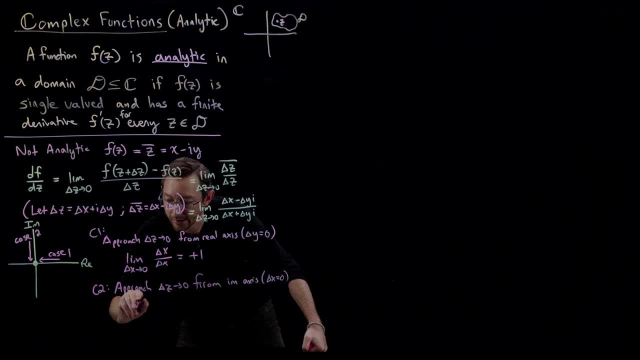 of delta y goes to zero. Now I have limit, delta y goes to zero. And now, remember, delta x starts at zero and I'm taking the limit of delta y goes to zero. But here I have minus delta yi over plus delta yi And if I take the limit as y goes to zero of this I get minus one. The i's cancel. 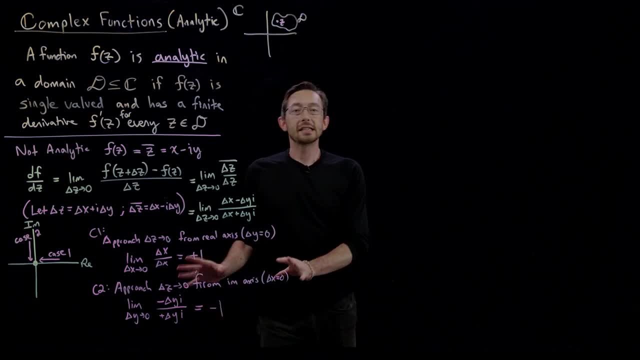 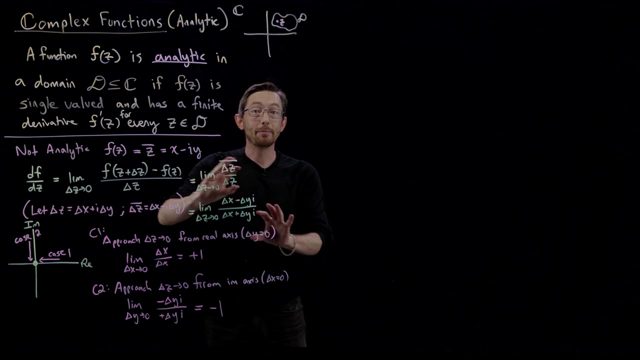 and the delta y's cancel and I get a minus one, And so this is super duper weird. okay, This function, the complex conjugate of z, the function f of z equals z bar, does not have a well-defined derivative. It does not have a derivative that is independent of the. 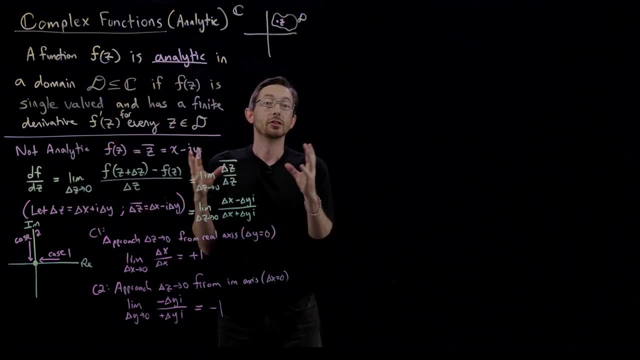 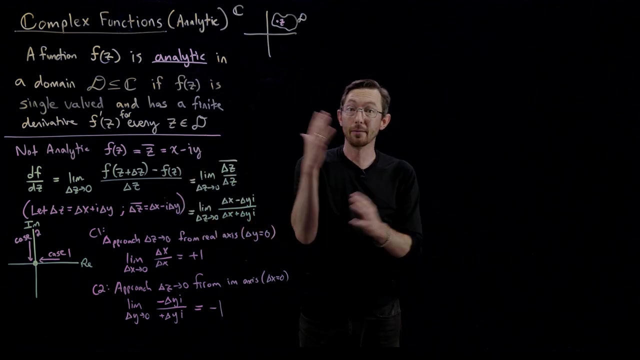 path of approach, that delta z goes to zero. So we know that this is the definition of a derivative, that the limit, as you know, my infinitesimal change goes to zero of the change in f over that change in z. But because these complex functions have a real part and an imaginary part I can take 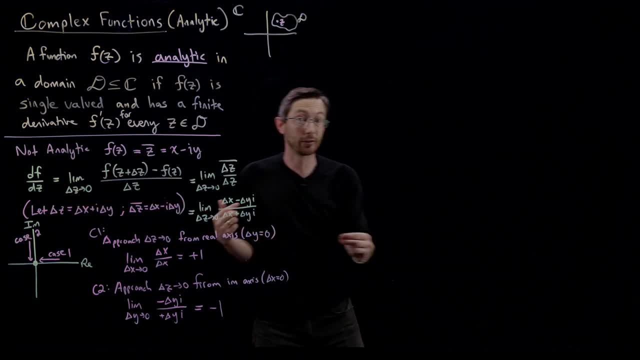 that limit, this derivative limit. I can take that limit approaching from the- you know- delta x direction or from the delta y direction. I can approach from any other angle and I'll get different derivatives. That's also super weird. I can approach from other directions, It's just. 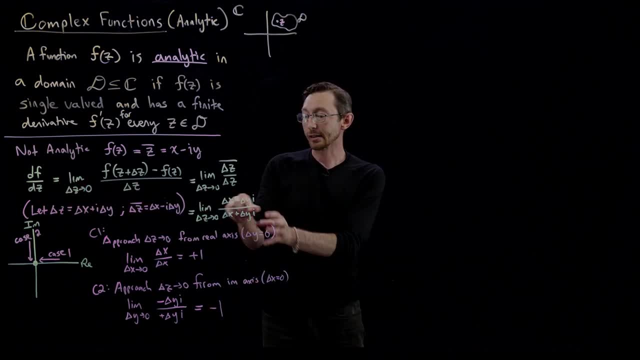 that these are the easy ones to compute And because of the way that this complex conjugate function works. if I approach from the delta x direction, I get plus one derivative. If I approach from the imaginary or the delta y direction, I get a minus one derivative. 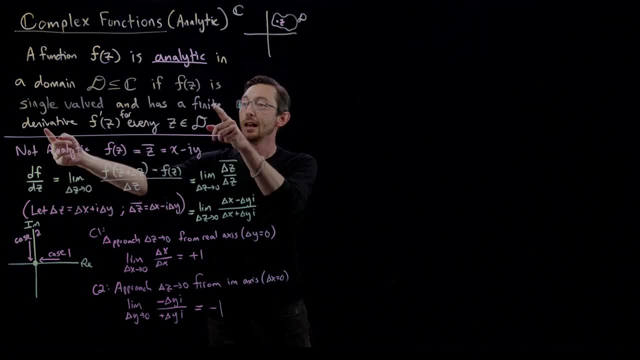 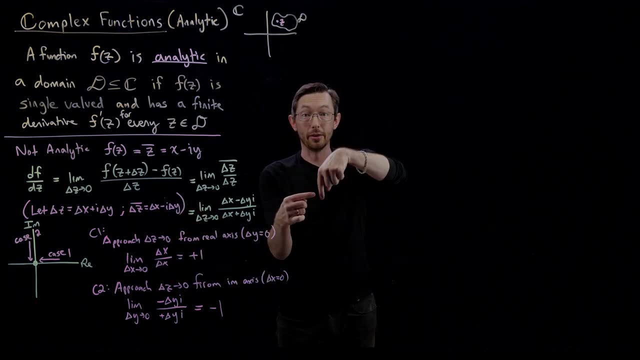 So this is not a. so this function does not have a well-defined derivative that exists at every z, Like it's. which one is it? This doesn't have a derivative. It depends on the path. So this is an ill-defined. 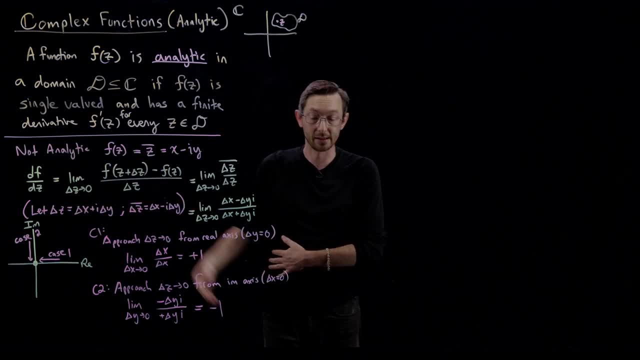 expression here. This is, you know, multi-valued. It doesn't exist. So this is a weird function that's not analytic and calculus is difficult because now the derivatives I take depend on the path I'm taking, okay, And so it doesn't have just an f, prime of z. I can't write df, dz. 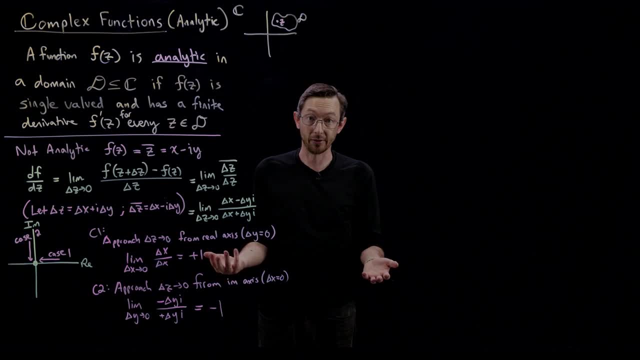 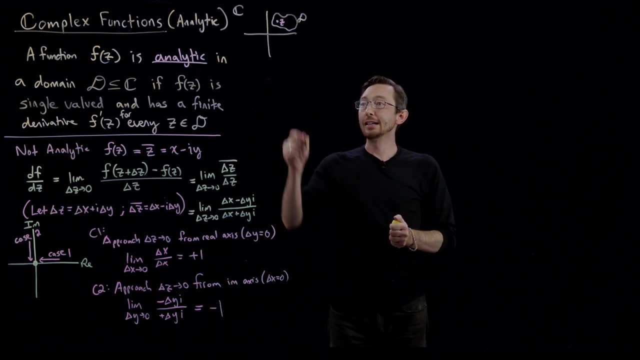 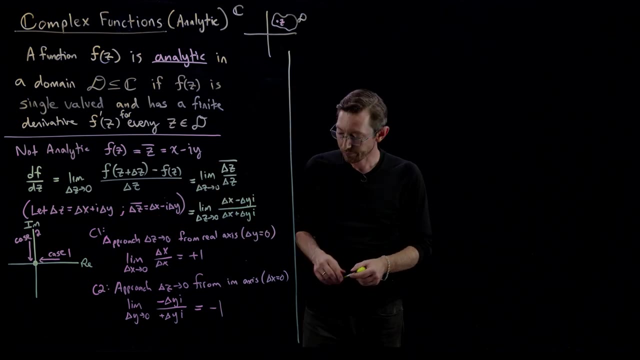 I have to specify which direction I'm taking. that derivative I need to. I can only specify directional derivatives for this function. Good, So that is a neat and kind of intuitive example of what can go wrong in the complex plane. So this is a non-analytic function, And so now I'm going to revisit. what does it mean? 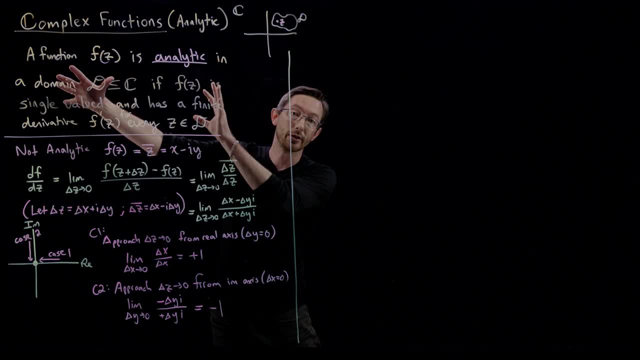 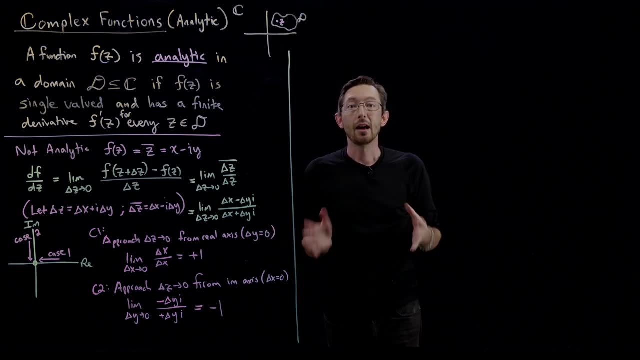 for a function to actually be analytic. So these are some conditions for a function to be analytic. Now we're going to start deriving. what are the outcomes, what are the kind of implications of that? And I will conclude by giving you some canonical examples of functions that yes. 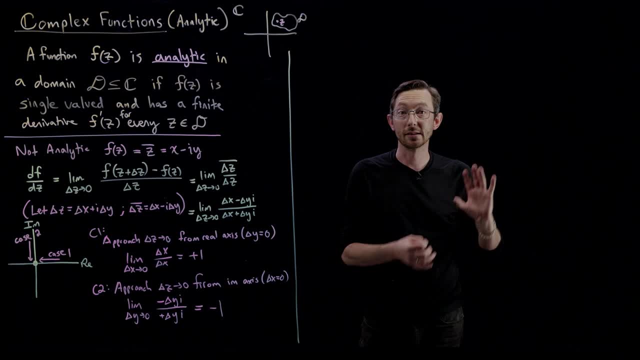 they are analytic, and some canonical examples of functions that, no, they are not analytic. okay, And I'm inclined, I'm almost feeling like I should just tell you some examples of functions that are analytic first. Maybe that's what I'll. 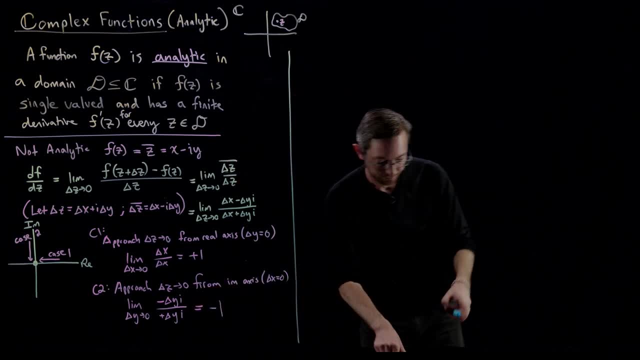 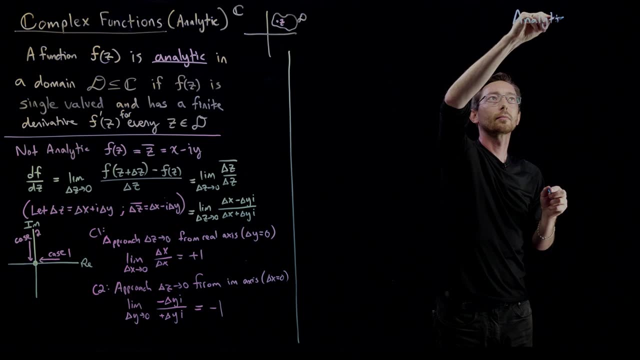 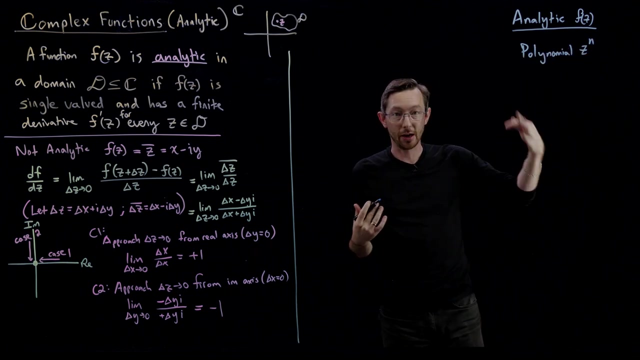 do, And I'll do those in blue. So I'll just do some functions that. yes, indeed, they are analytic. So analytic functions, analytic f of z would be things like any polynomial. So polynomials, Z to the n for integer n, for, you know, n equals 1,, 2, 3, dot, dot, dot. okay, Not for n equals. 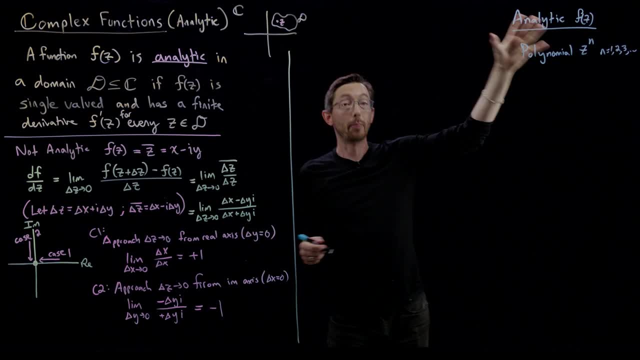 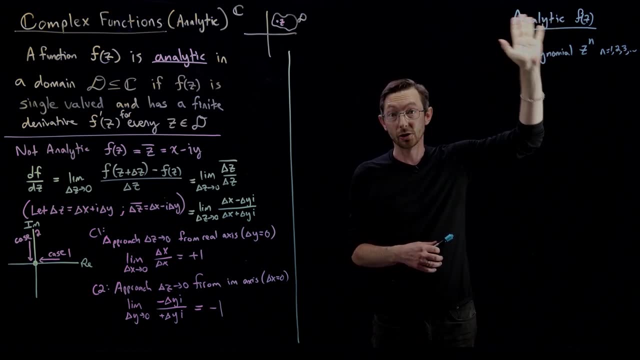 one-half or one-third or one-quarter, because those are not single-valued Polynomials, monomials, you know, sums of monomials, polynomials, things like that. Those are in fact analytic functions. Yes, indeed, they are analytic, Maybe at the very end of this video. 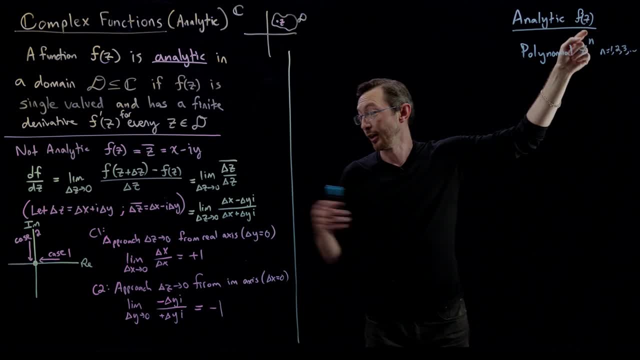 if I remember, I'll just take the polynomial z and we'll do this exact same limit and I'll confirm for you that, yes, in fact it satisfies this property that the derivative does not depend on the direction. So I'll probably put chapters. 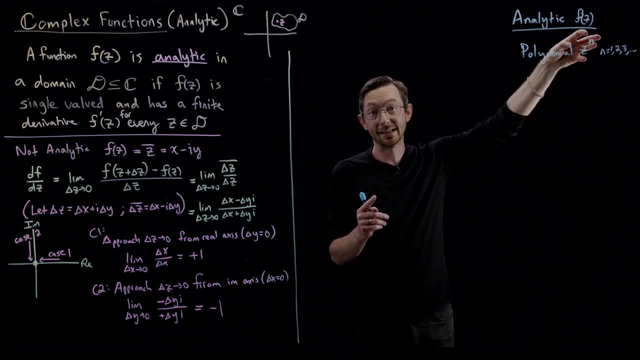 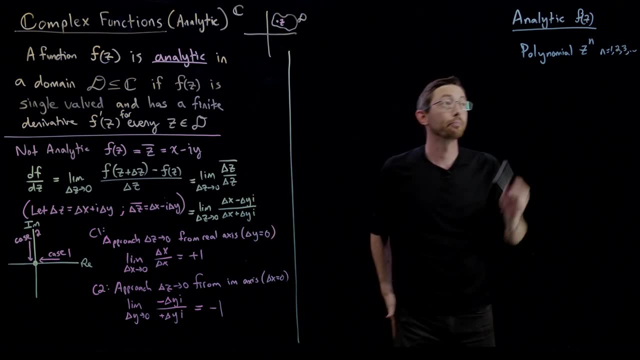 in this video, and you can fast-forward if you want to see me derive that, yes, z squared is in fact analytic and that the directional derivatives equal each other, no matter what direction I come in from. Polynomials, other functions, that are good ones. So this is kind. 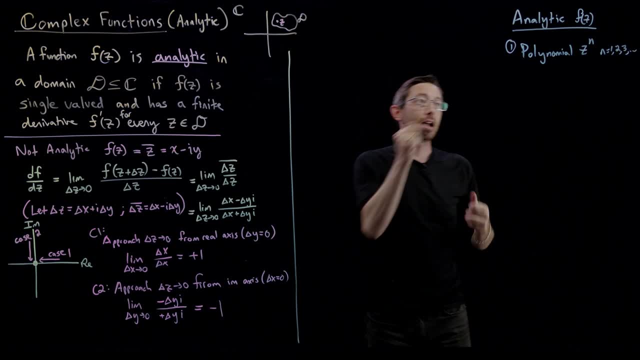 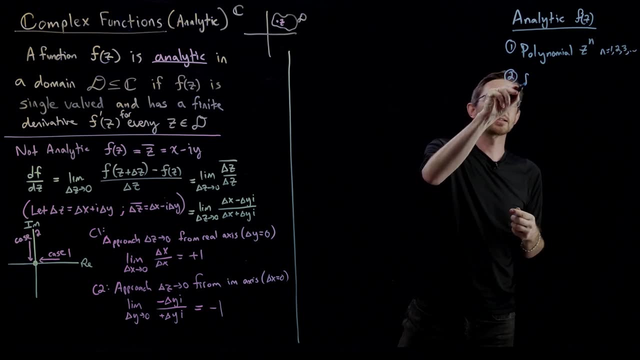 of one huge class. Another big class- and I'm not going to go through all of them, but I'm going to go through all of them. So this is kind of one huge class. Another big class are functions, where the Taylor series exists. That's kind of a vague way of saying it, but I'm just going to say 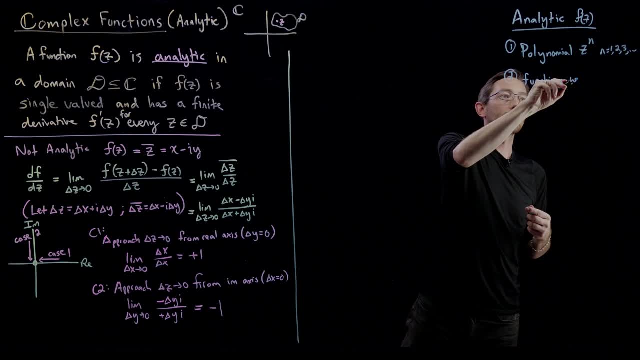 functions kind of with a Taylor series, a well-defined convergent Taylor series, And those would be functions like you know, e to the z or cosine of z or sine of z. We know that these are convergent functions. They have a convergent Taylor series for all points. 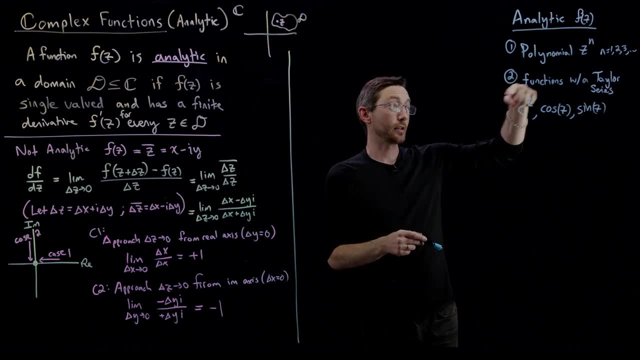 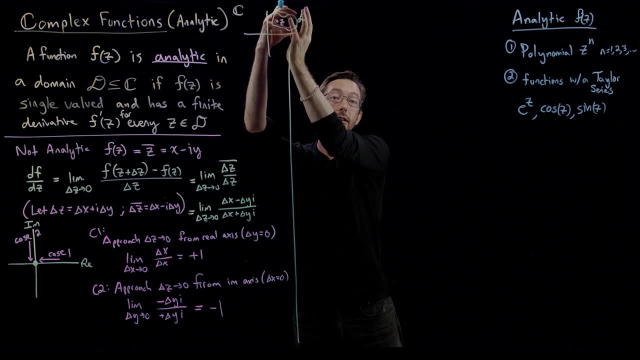 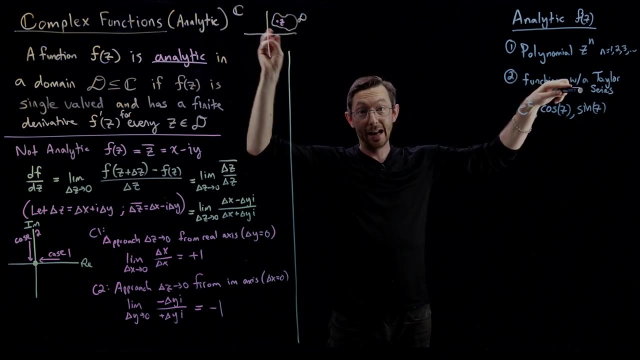 z in the complex plane. In fact, these functions polynomials and e to the z, cosine of z, sine of z. these are not just analytic in some small neighborhood d, They're analytic everywhere in the complex plane, For every single point z you can name. these are analytic at every point. 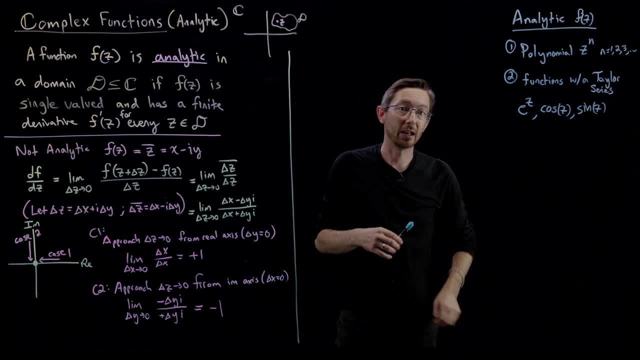 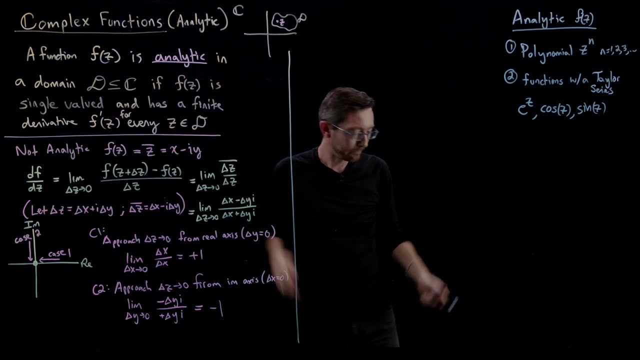 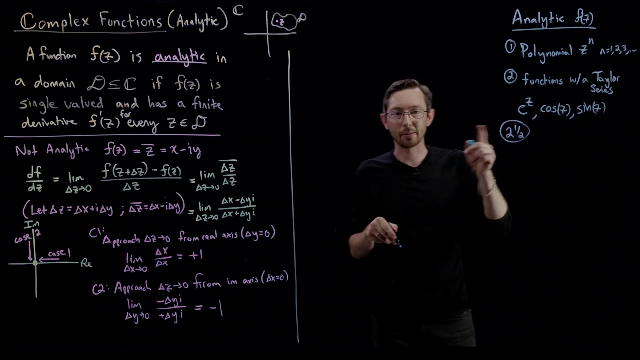 which again I told you in a previous lecture, the name for that in complex analysis and mathematics is called an entire function. if it's analytic everywhere, Okay, if you can do calculus absolutely everywhere, And then actually there's kind of a fun kind of two-and-a-half case where this is like platform. 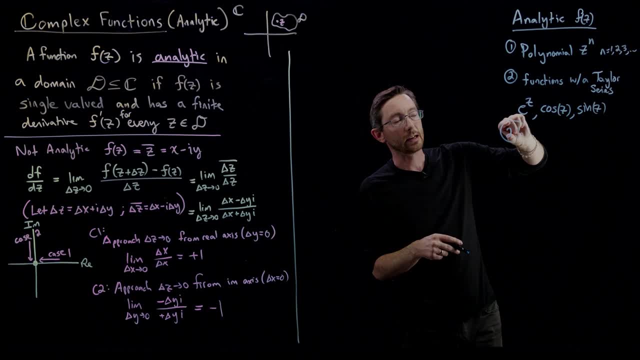 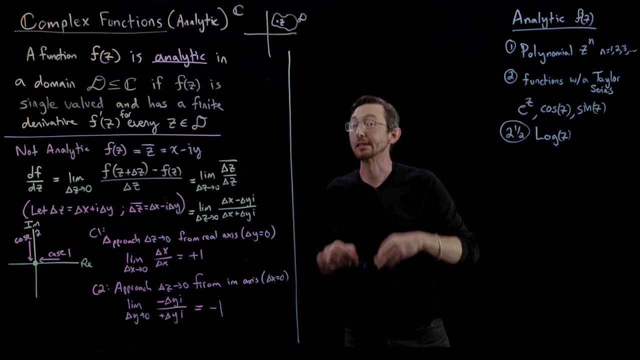 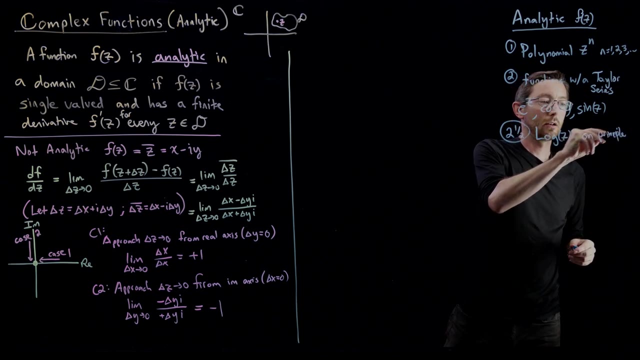 nine-and-three-quarters, So this is kind of a halfway case. The log of z, okay, the log of z on its principal branch, you know, on principal branch. let's hope this doesn't on its principal branch. so remember this function. the imaginary part. 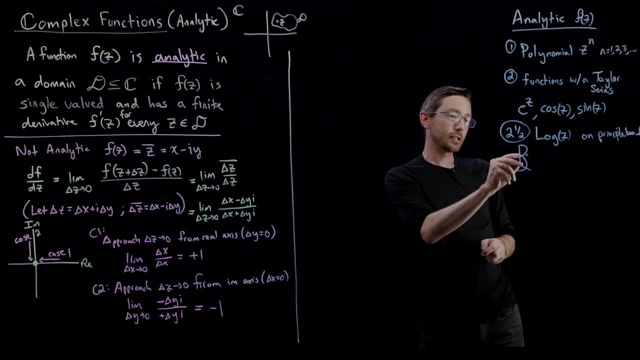 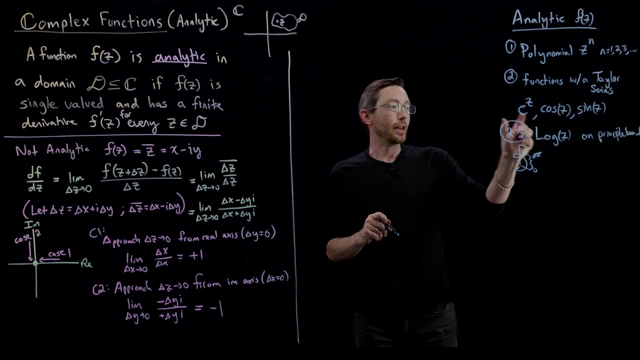 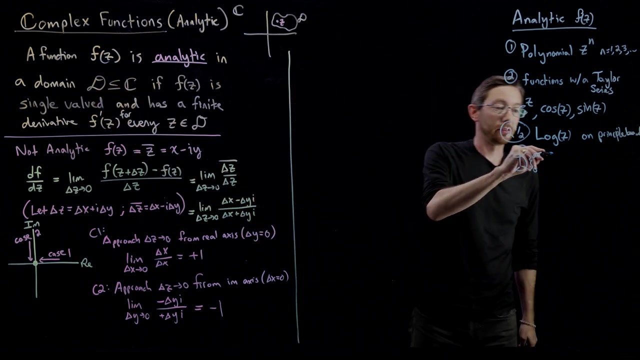 kind of forms, this spiral staircase. If I just take the first branch of this thing that goes from zero to two pi, then that log of z is single-valued on that branch. So if I only define the log of z on that principal branch then that is actually analytic everywhere except at z equals zero. So 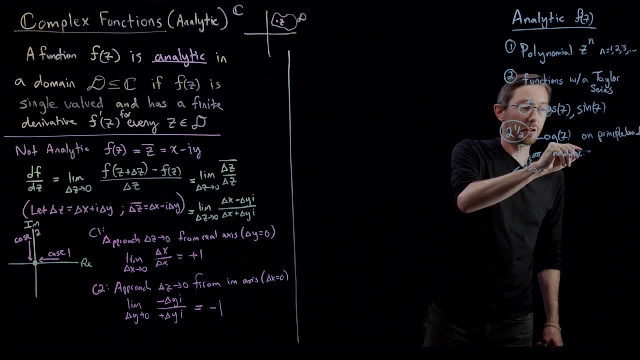 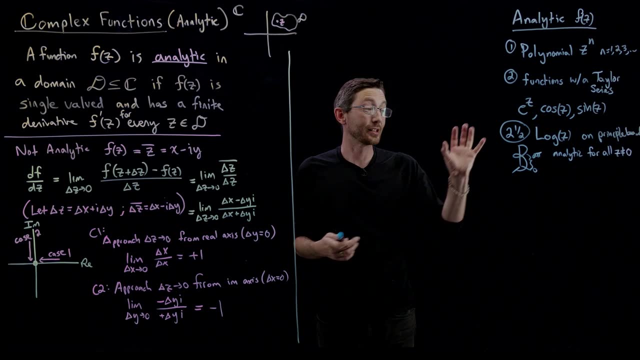 this is analytic for all z not equal to zero. Okay, so it's analytic almost everywhere. It's not an entire function. It does have this weird non-analytic point at the origin. So if I do a contour, integral around that point, 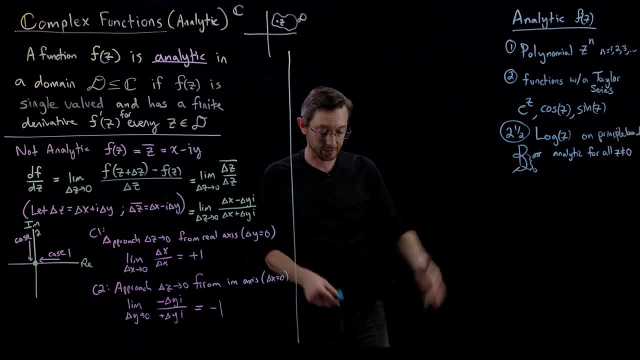 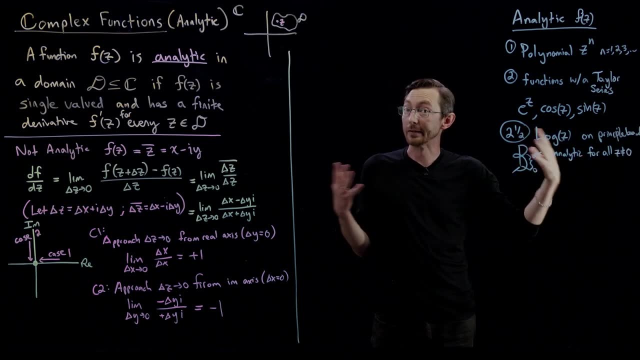 weird things will happen and I'm going to show you that in this lecture at the end, and in the next lecture And in probably all of the next five lectures we're going to talk about. you know, that single weird point where this is not analytic is very important, But it's analytic. 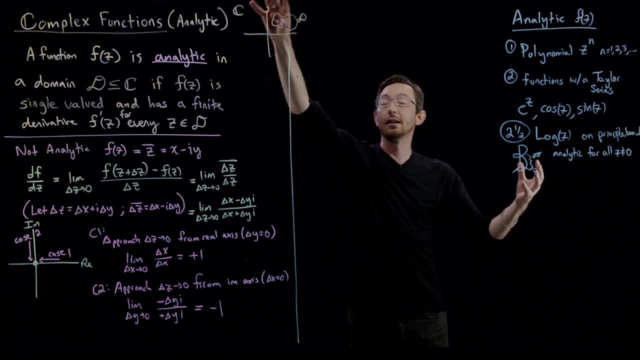 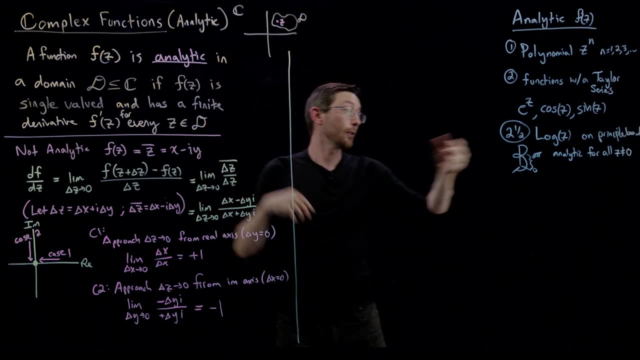 almost everywhere It's analytic on large swaths of large domains of the complex plane that don't encompass that origin. So in fact, this place, this domain that I drew here- log of z- is analytic on that domain. if I'm only considering the, 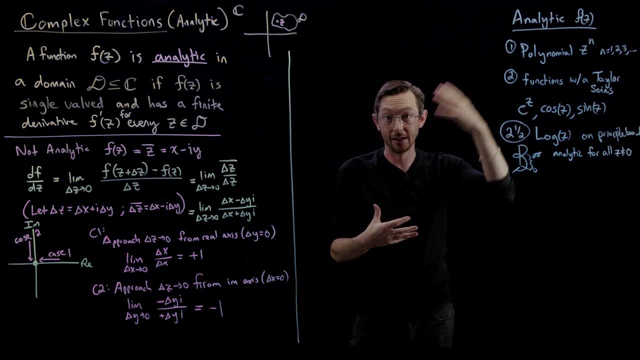 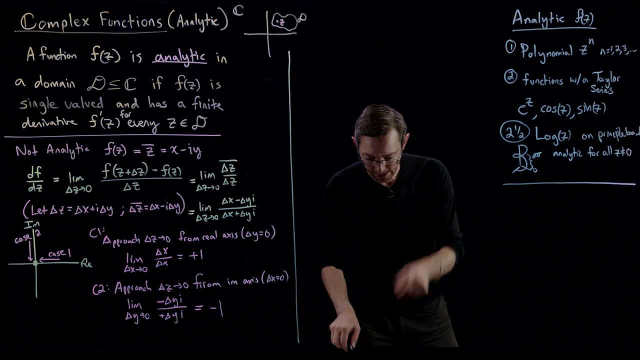 principal branch that goes, you know, up one flight of that spiral, that infinite spiral staircase. So these are functions that, yes, indeed, they are analytic. And now I'll just give you a few examples of weird functions that are not analytic. So not analytic. 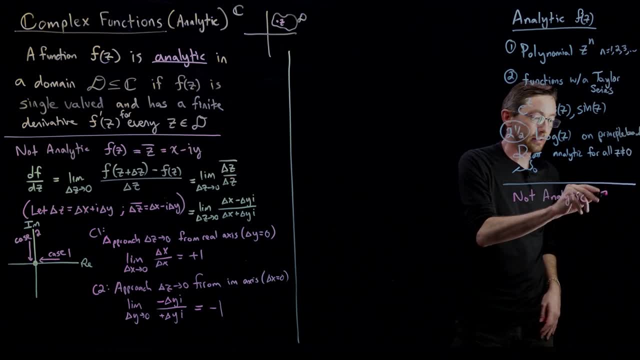 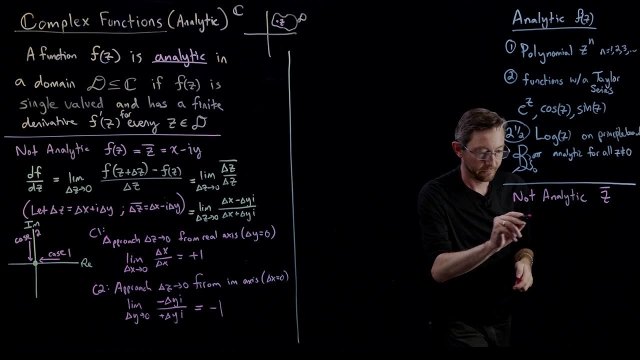 Would be things like, you know, z bar. So things like z bar where the derivative is different at different directions, So anything that has a singularity, So any function that has kind of a singularity, where this, you know, goes to negative infinity. So any singularity the function is not. 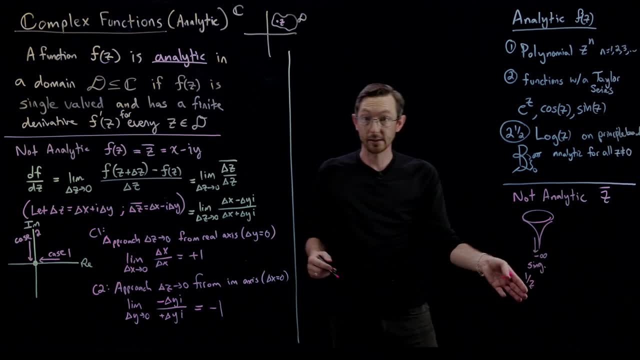 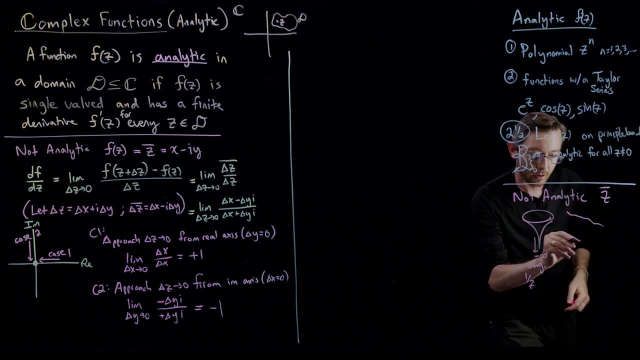 analytic at a singularity. So things like one over z are going to give us lots of trouble If I have a cliff, if I have like a cliff in my complex landscape. so you know, I'm from Texas and in Texas we have the Lano Escarpment in West Texas where, if you approach at this, 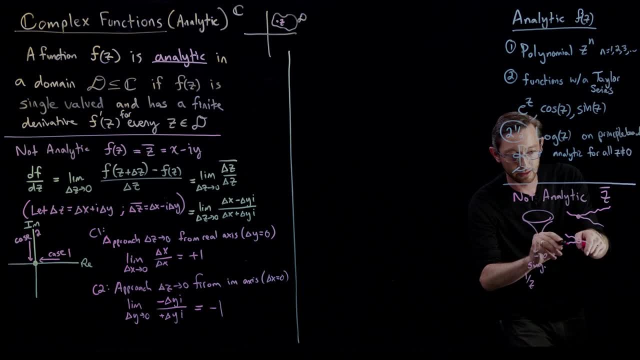 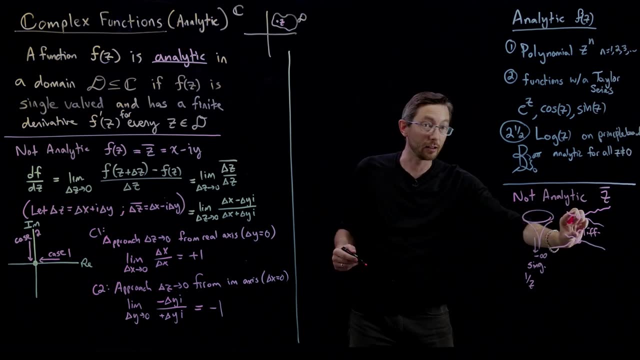 point. it kind of drops off maybe a thousand meters and there's a cliff. So cliffs are not analytic because the derivative would be infinite at that cliff and it would not exist. It would not have a finite derivative at that cliff. Okay, The function log, if I don't consider it on this, 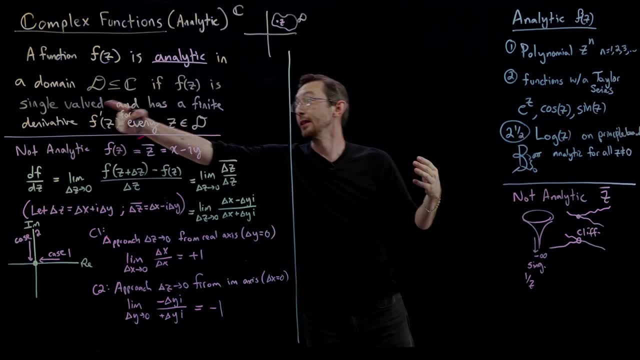 principal branch is also not analytic because it would be infinitely valued. The function z to the one half is not analytic because it's infinite. It's not infinitely valued. It has two values. It's not single valued Cusps. also, if I have a function, 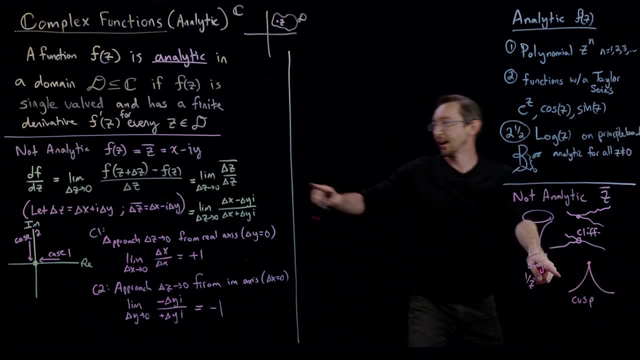 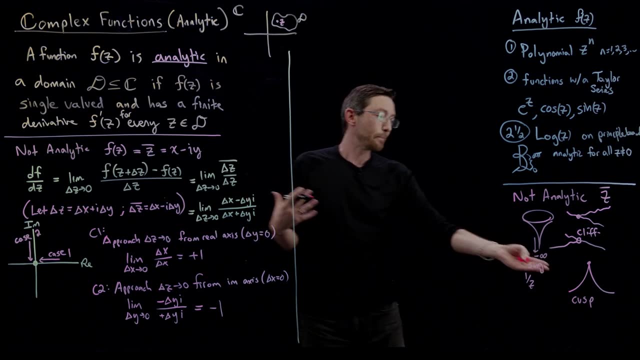 that has a really sharp cusp and in fact kind of z bar. if you, you might actually want to fire up MATLAB or Python and plot the real and the imaginary parts and you'll see that this function is actually a bit cuspy. And that's kind of a weird thing, is that it's cuspy depending on. 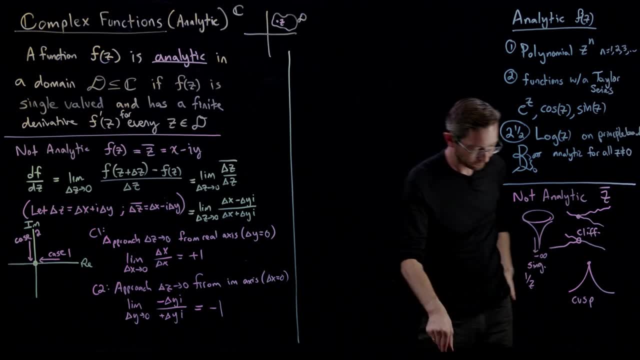 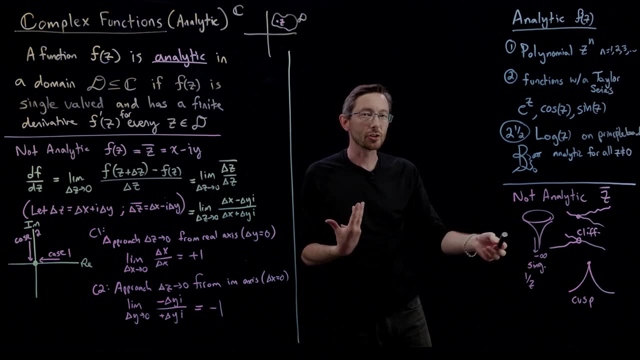 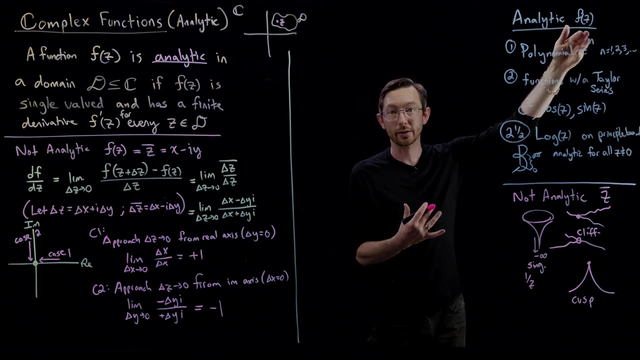 what you know, direction you approach the function, And kind of my rule of thumb for not analytic functions is it tends to be functions that cannot easily be represented as a closed form of z. So z to the n is kind of only written in terms of z. 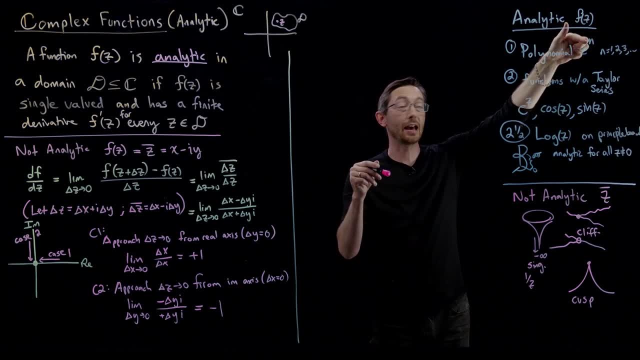 and if I did f prime it would be n? z to the n minus one. That's like a well-defined derivative, Same with e to the z cosine, z sine of z. But z bar can't be defined as a primitive function of z, It can only be defined-. Can you spell it for me, Z, I don't know You could spell the 12 minus 1말iRun was execute d f, prime of the tone z bar can't define as a primitive function of z. Again, if you look at the sin, 맛있 and the maneira, but the 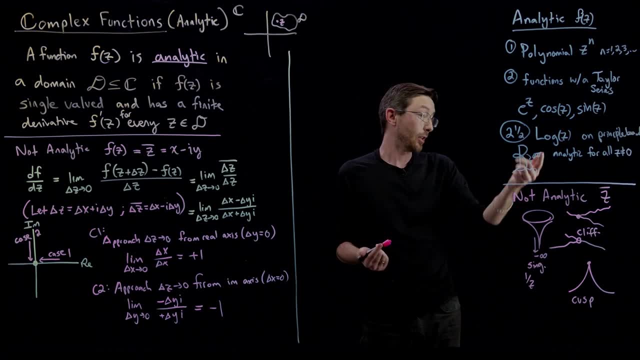 terms or theirmiading, you can really see that the function or the derivative in the Poisson in terms of the real and the imaginary parts of z, Same with logarithm. actually, right, We can't really write log of z as some primitive expansion of z. 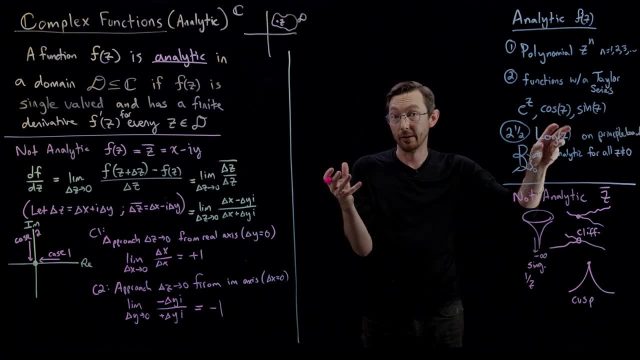 We need to write it in terms of the real and the imaginary, or the magnitude and the phase of z, And so that's kind of another rule of thumb I use is, if my function can't be written as a simple function of z, but I need the real and the imaginary parts to specify this. 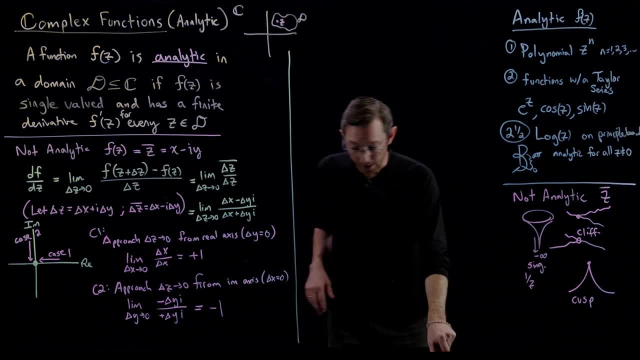 usually those functions are not analytic. Okay, good, And again, as a general rule of thumb, if I just randomly pick a complex function out of a hat, chances are 99.9999999% of the time it's not gonna be an analytic function. 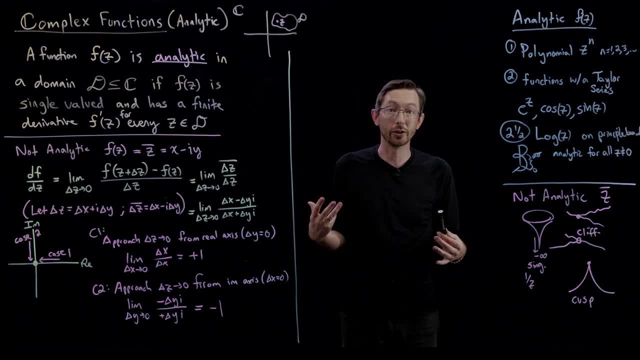 The vast majority of functions. if I just randomly generate a function in the complex plane, it's not gonna be analytic. So analytic functions are very, very special. In math we call this measure zero. They're a measure zero set in the space of all functions. 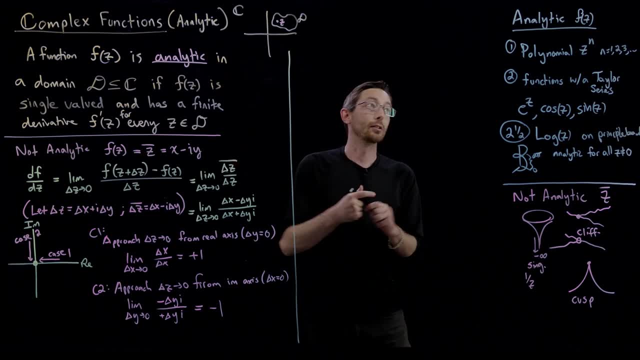 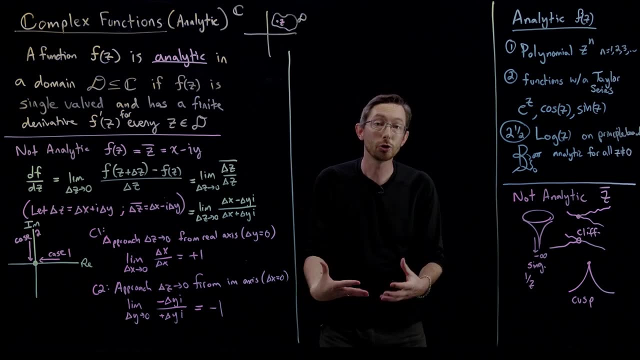 They're extremely rare, special functions where you can do cancels, You can do calculus, Good, Okay. so now what I'm going to do is I'm going to derive the Cauchy-Riemann conditions for a function to be analytic. 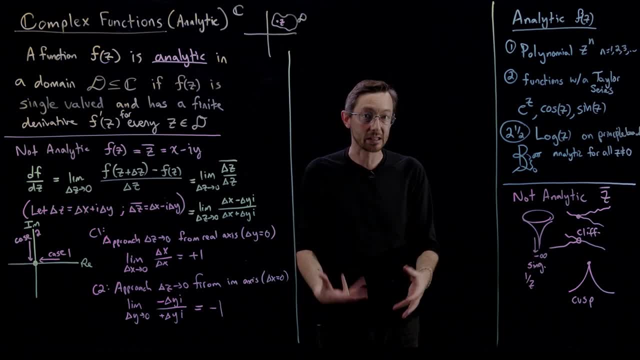 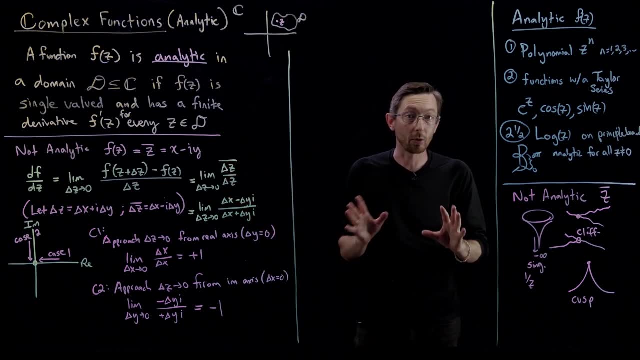 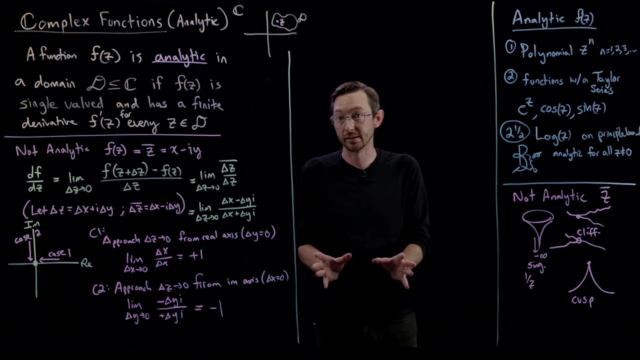 And this is in terms of partial derivatives. It's an extremely powerful expression in math and it ties these complex functions to partial derivatives. It's one of the most important conditions or relationships in all of complex analysis. It's kind of one of the cornerstones of complex analysis. 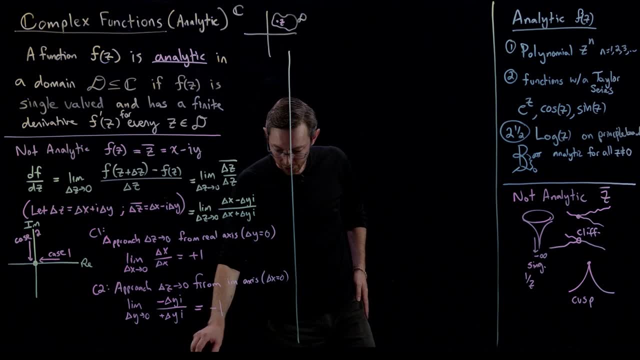 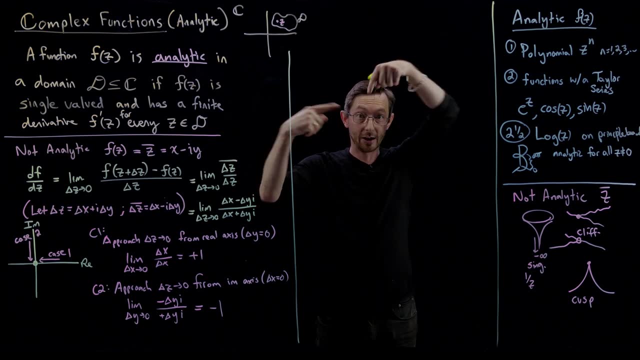 So this is super important. So the Cauchy-Riemann conditions are very important. For a function to be analytic, we need for its derivative to be the same, no matter what direction I approach that derivative. So I'm going to write this out. 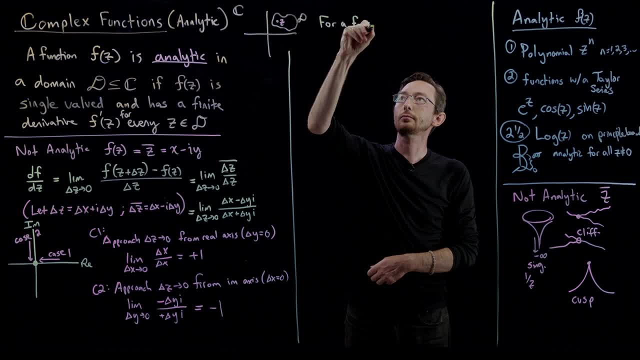 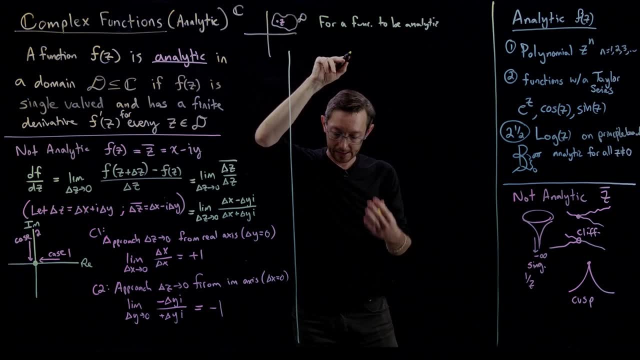 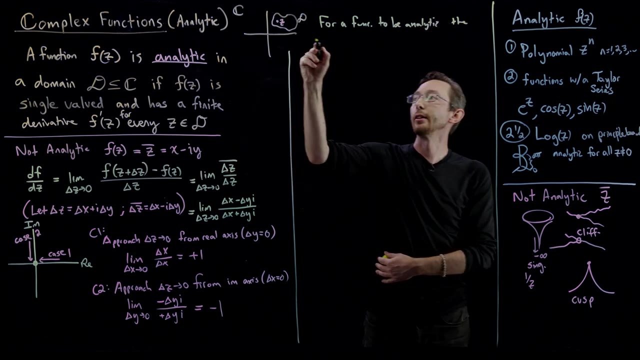 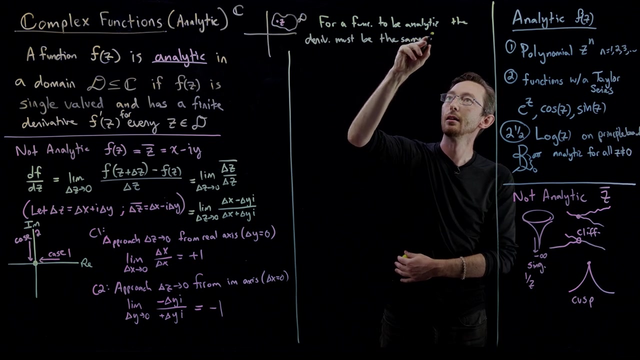 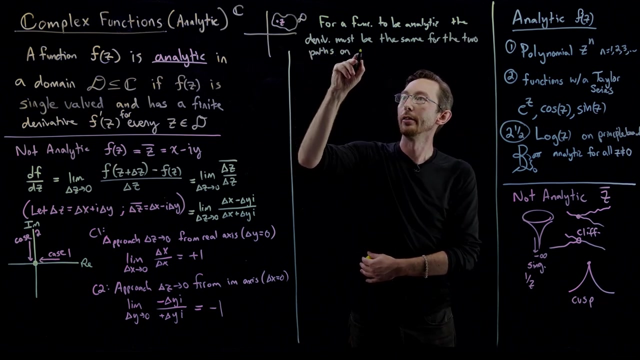 For a function to be analytic, the derivative must be the same of the two paths taken on the real and imaginary axes. For a function to be analytic, the derivative must be the same of the two paths taken on the real and imaginary axes. function be analytic, the derivative must be the same for the two paths on the. 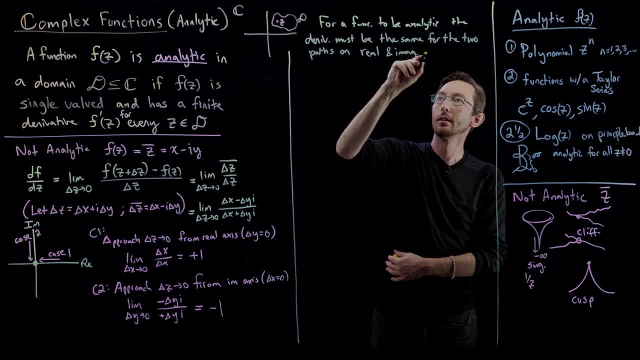 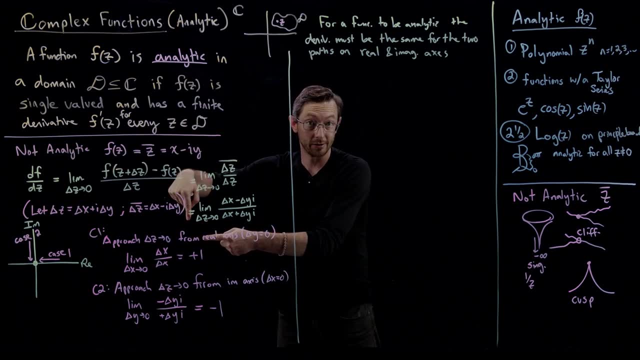 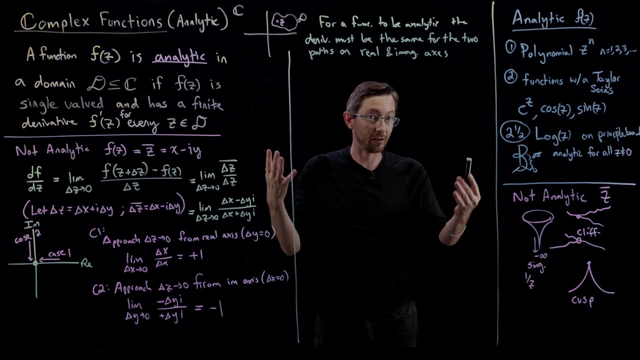 real and imaginary axes, kind of what I drew down here: the, if I take my derivative in, the Delta X goes to zero direction or the Delta Y, it goes to zero direction. those have to be equal. now this you would need to do some proof you. this is a theorem. you would need to prove that theorem, that if this is true, 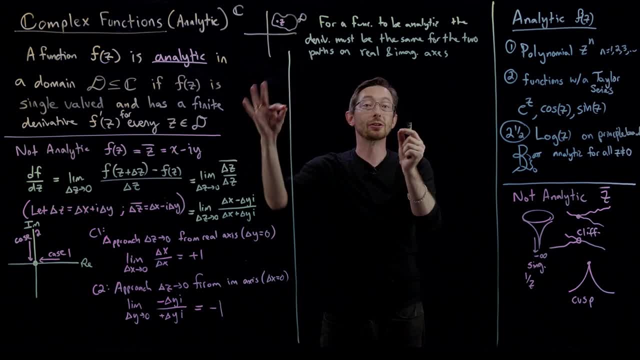 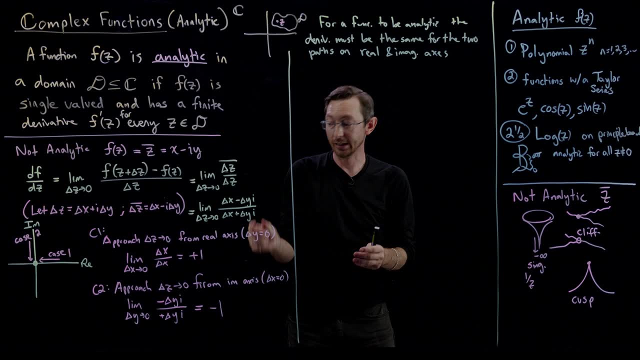 if these are equal on the real and the imaginary axes, then it's real from any approach angle. for any way that I could possibly approach, Delta Z goes to zero. if the Delta X limit equals the Delta Y limit, then this is true for any approach angle: Delta Z goes to zero. that's something you would need to prove. 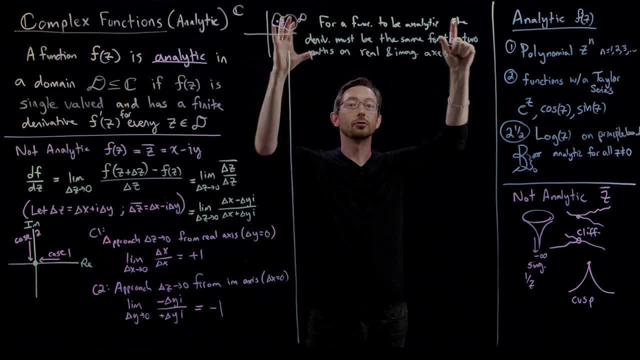 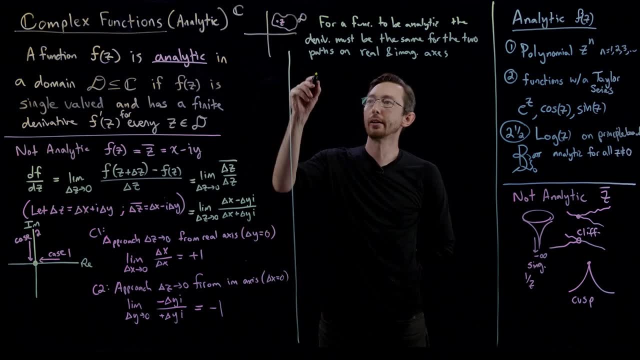 I'm just going to. we're going to say, if that's true, then this function is analytic. that's kind of the Cauchy-Riemann hypothesis. and so what we're going to do is we're going to define our, you know, F of Z equals. it has. 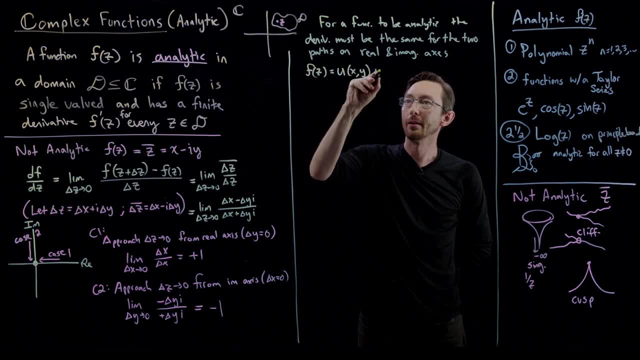 a real part U of X comma Y and an imaginary part I of V of X comma Y, where you know, of course, Z equals X plus I, Y. okay, so this is going to be the function we're going to take. the derivative of it has a real part and an imaginary part. 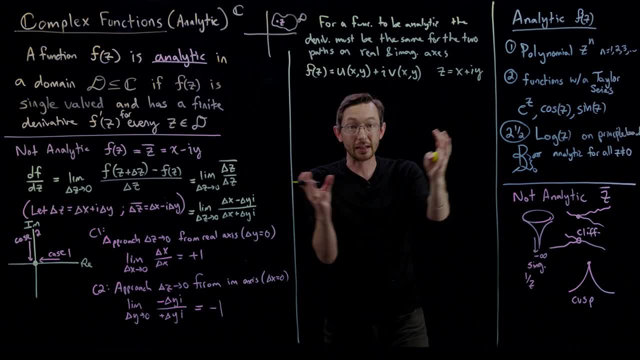 and this is the Z that we're going to take. the infinitesimal limit of Delta Z goes to zero, okay, which means we're going to take Delta X goes to zero, Delta Y goes to zero and we're going to kind of derive what conditions have to be. 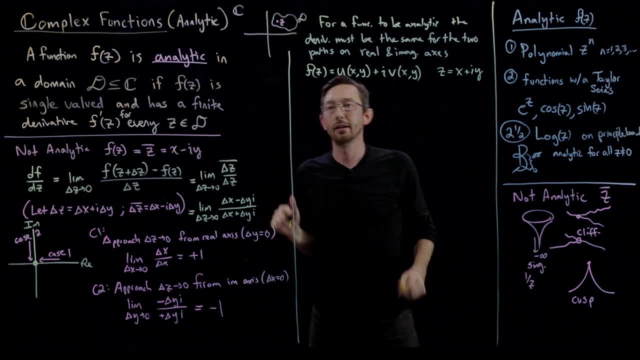 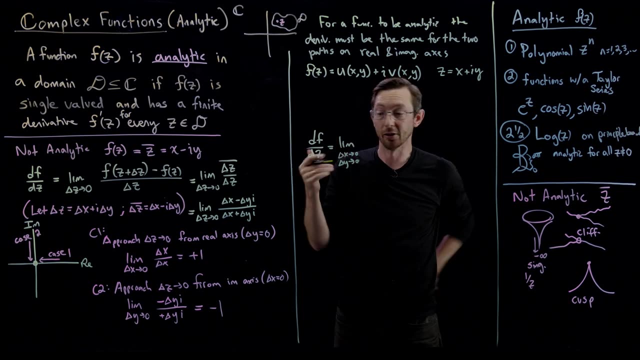 true, and I'm gonna give myself a little room for my head. so d realizaralta yo está bien, exactamente como escribimos aquí. está la r? Düna después del. Delta X va al zero, y to zero. that's the same as saying delta z goes to zero. both of these have to go to zero. they. 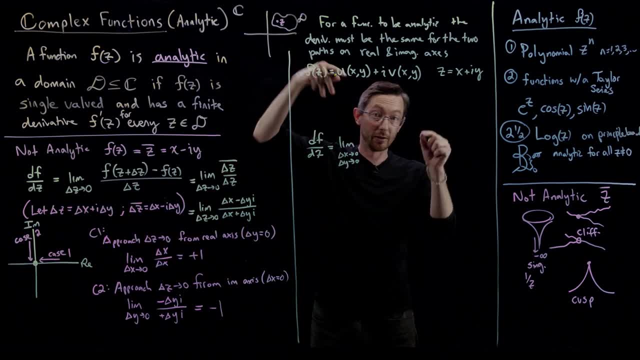 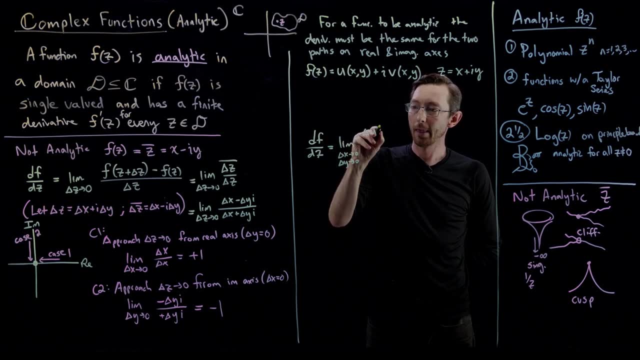 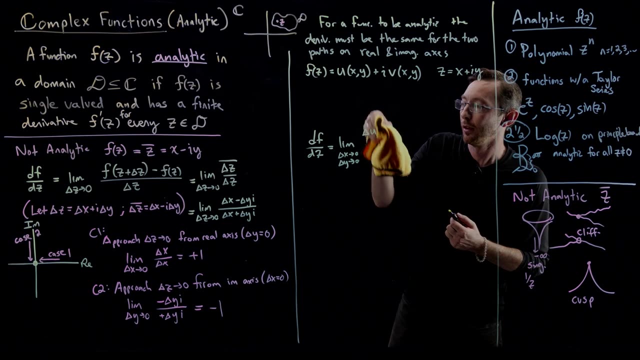 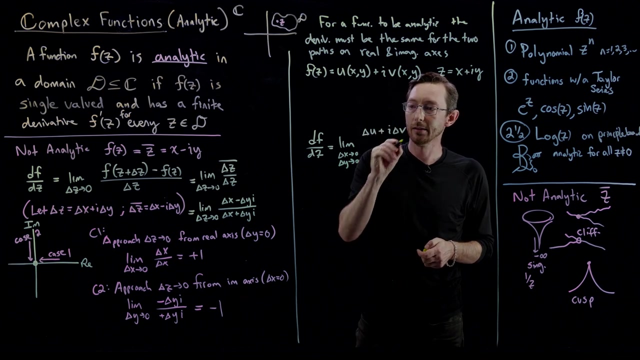 could start at zero, as in these two cases, or they could start both non-zero and go to zero, any way we like. of delta u of, well, let's say delta u. it could be of course it's delta u of x comma y. but let's just say delta u, delta u plus i, delta v divided by delta x plus i, delta y. again you can. 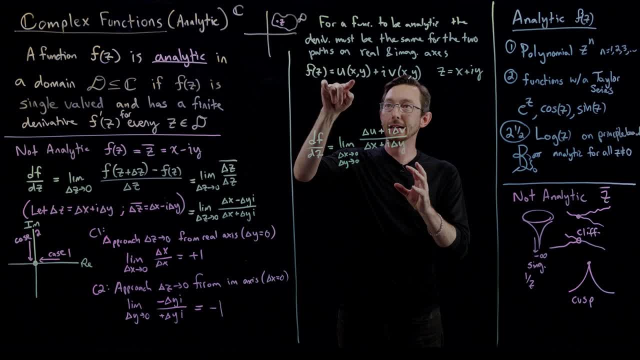 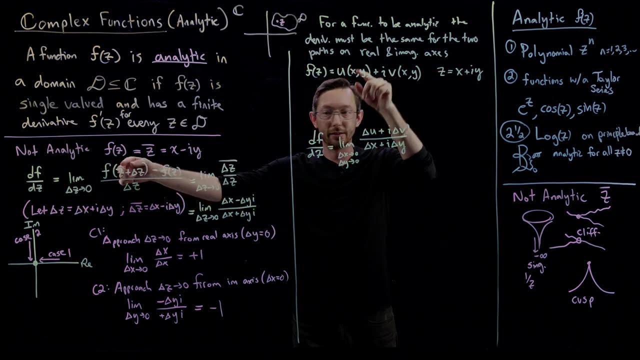 pause the video and, you know, actually plug in x plus delta, x, y plus delta y. you know, v of x plus delta, x, y plus delta y, and you know expand that out in a first and final order and then you can use the first order, taylor, series, and, and, uh, you know, cancel out the f of. you know, like the the. 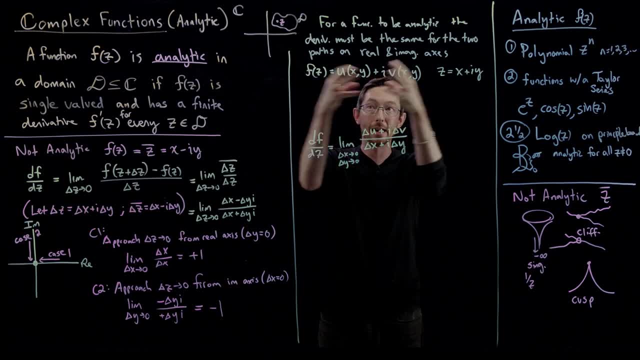 terms that are not plus delta z, and this is what you're going to be left with. so you can expand that out in a taylor series: f of z plus delta z. expand that out. subtract f of z, and this is what you're going to be left with up to first order, and we're going to again divide by delta z. okay, so you. 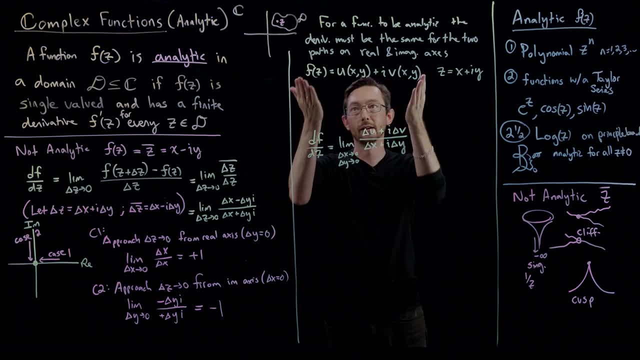 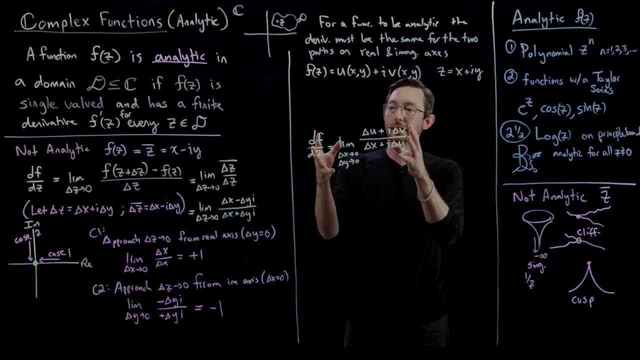 can pause and verify that. this is what you get, uh, when you plug this into this expression and use the taylor series. and now what we're going to do is we're going to go back to the first order, and we're going to do is we're going to take this and again, we're going to take it approaching from. 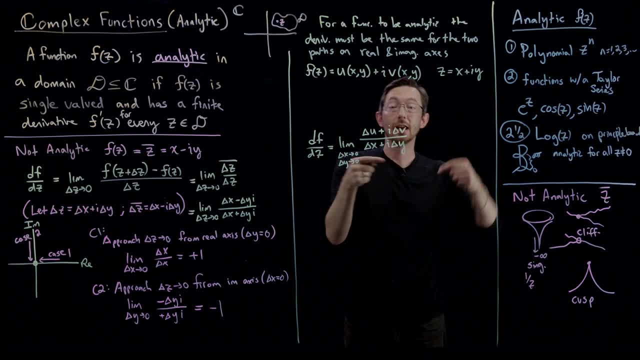 the real axis from the delta x goes to zero direction and from the imaginary axis, from the delta y goes to zero axis and those have to be equal for this to be an analytic function. so kind of you know approach. one again is kind of on the real axis. 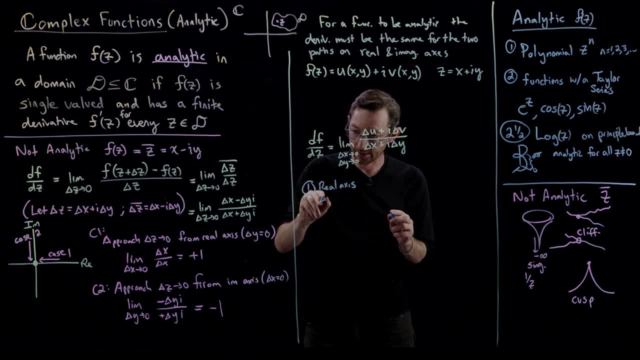 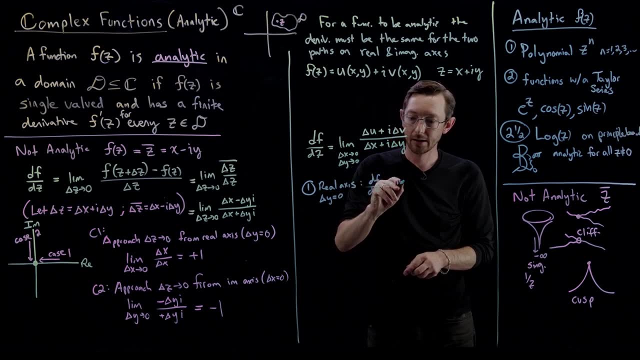 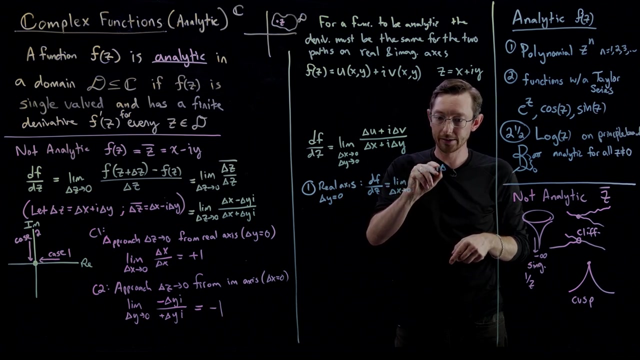 which is the delta y starts out being equal to zero, and we say df, dz equals limit, as delta x goes to zero. delta y was already zero because we're starting on the real axis. delta x goes to zero, the limit of um, delta u plus i, delta v over delta x. now this is kind of 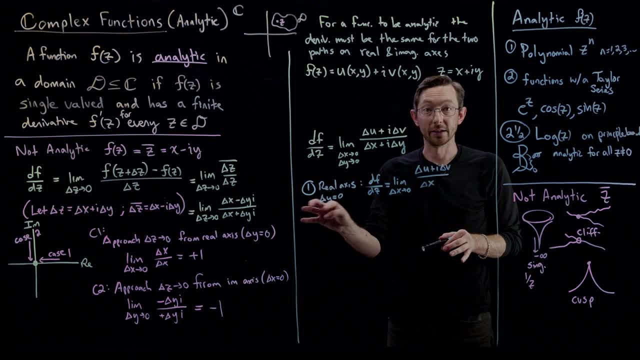 fun because we froze y equals zero, delta y equals zero and we're approaching on the real axis. this derivative here is actually a partial derivative. the limit is as delta x goes to zero for y frozen of delta u over delta x, that's the partial of u with 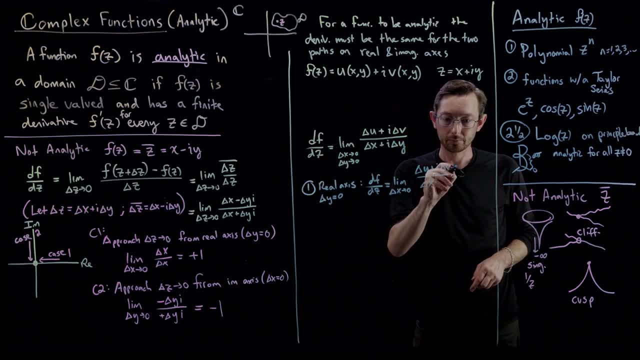 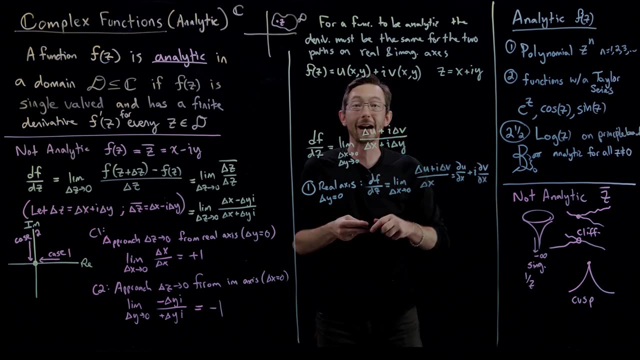 respect to x. so this is um, partial u, partial x plus i, partial v, partial x. this is super important. so i'm going to put a little. you know i'm gonna. well, maybe i'll bracket that in a minute. this is super important. so if i take the derivative on the real axis of this function, i'm going to put: 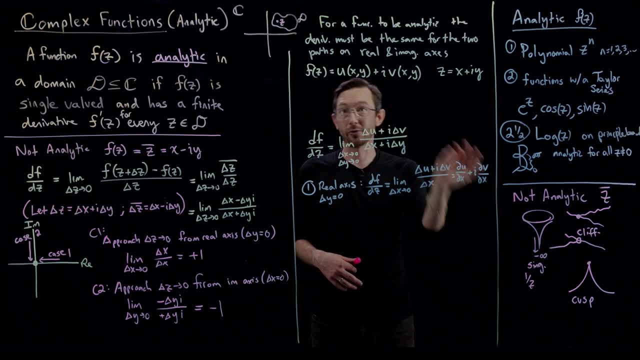 the derivative on the real axis of this function, i get partial u, partial x plus i, partial v, partial x, for whatever u and v happen to be. this is going to be what that derivative is. in fact, you can verify, you know here, f of z, u is x and v is minus y, and so you can actually. 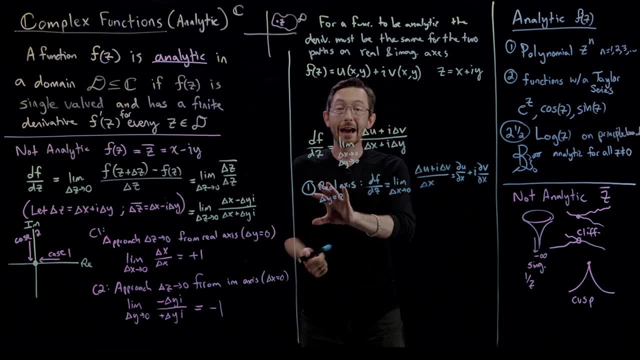 compute what these are, if you like. and now we're going to compute what is the derivative if i approached on the imaginary axis. if i froze, delta x equals zero. so now what we're going to do is we're going to approach on the imaginary axis as if delta x was frozen on the imaginary axis. 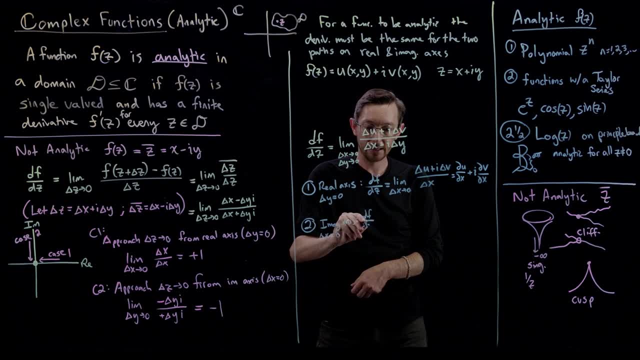 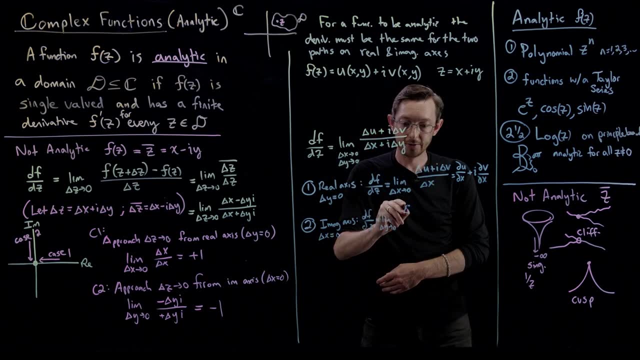 frozen at zero, and so d, f, d, z equals limit as delta y goes to zero. now delta y goes to zero of delta u plus i delta v. over now we have an i delta y. okay, good, and these two expressions are going to have to be equal for that function to be analytic. so we're going to use, we're going to take. 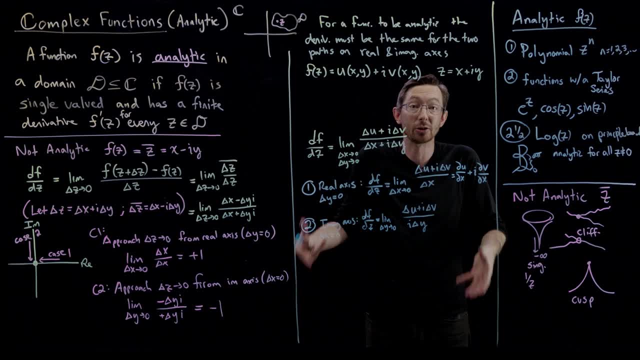 these and set them equal to each other and derive a set of conditions that has to be true for that function to be analytic. that's where we're going with this, and now you kind of see this funny thing that's going to happen because i'm dividing by i. 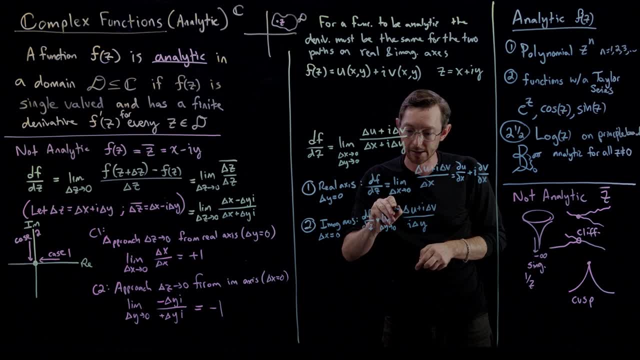 if you like, i can multiply top and bottom by- uh, let's say i times i and um. if i multiply top and bottom by i times i, i'm going to get some pluses and some minuses and some weird stuff. i'll just write down what happens, so i'm going to get you know this is going to be a partial u, partial y. 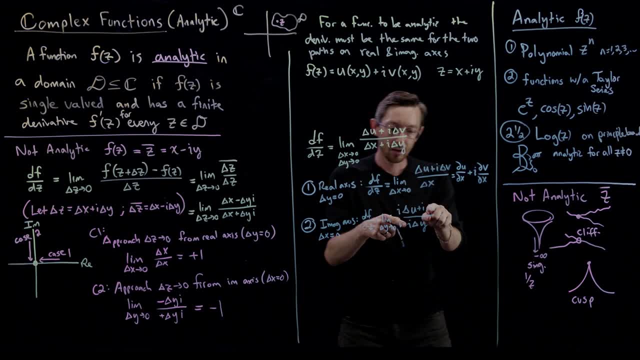 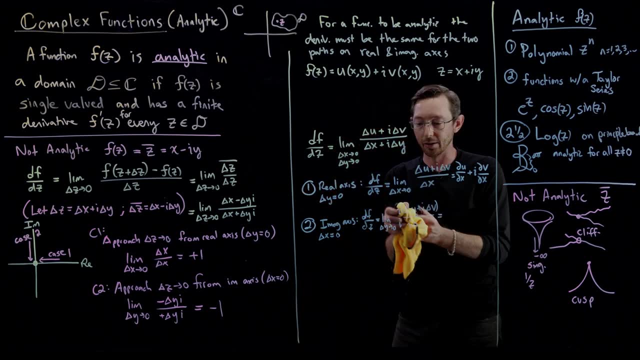 so that's a partial u, partial y, but it has an i out front. here i times i. i'm going to- i don't want to like confuse everybody- i'm going to multiply each top and bottom by i, and so this becomes a minus one. so this is a minus, and here this i delta u. 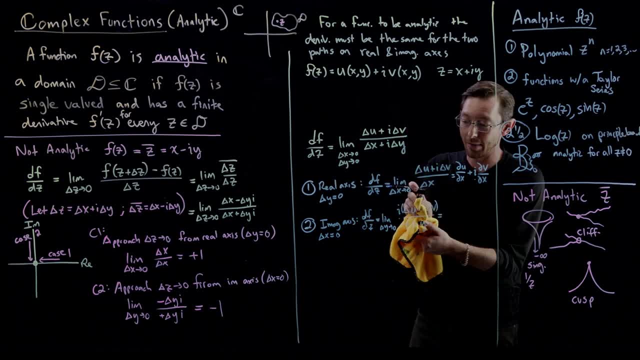 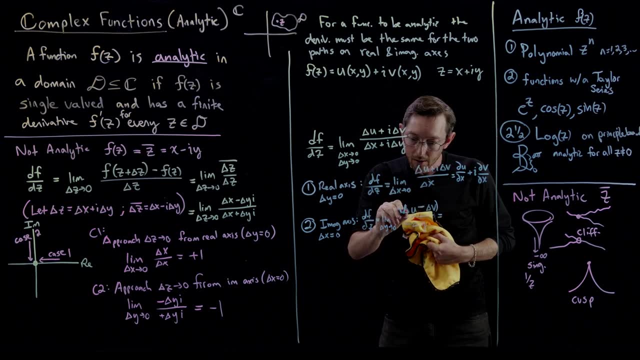 becomes i delta u, and this i times i delta v becomes minus delta v. so i have i delta u minus delta v. that's what happens when i divide by i. apparently okay, remember, because limit the, the delta y, had an i out front. and so now, if i take 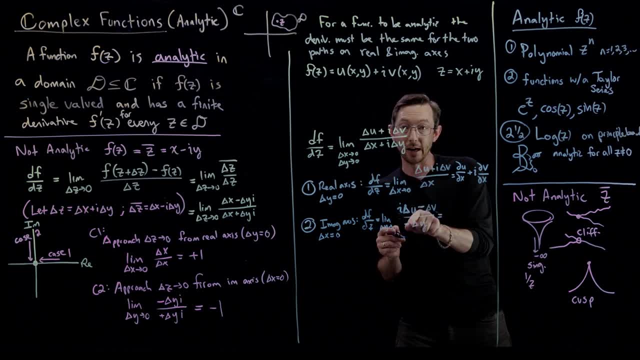 the partial derivatives. the real thing is minus partial v over minus partial y. that's just partial v, partial y, and the imaginary part is going to be again: minus i, partial u, partial y, partial u, partial y. okay, so that was a lot again. what we're trying to do here is we're going to 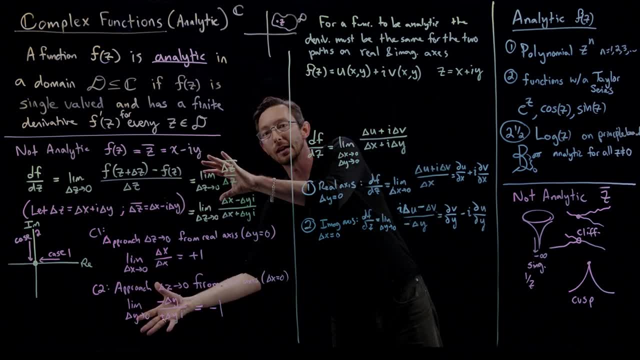 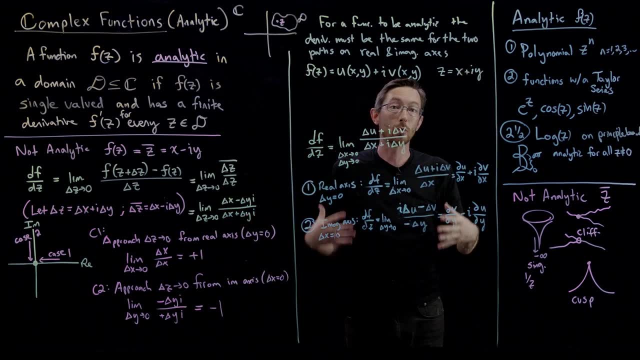 do is we're trying to- uh, essentially we- we showed the example of what weird thing can happen when you approach from different directions and have a non-analytic function when they don't equal. so we're trying to derive conditions for what has to be true for the real and imaginary part of my 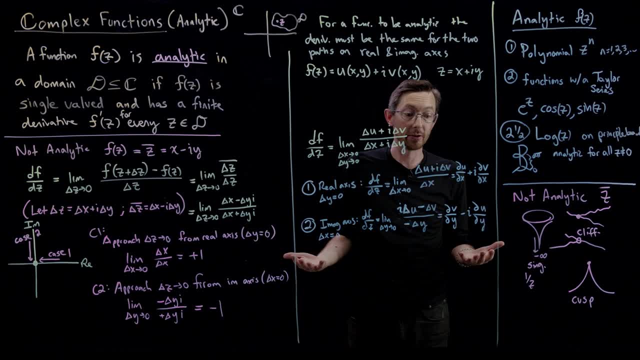 function for these two directional derivatives to be equal to each other. and the two directional derivatives, if i approach on the real or the imaginary axis, are these two partial derivatives of u and v. and so now, what we're going to do is we're going to equate the real parts of these, the 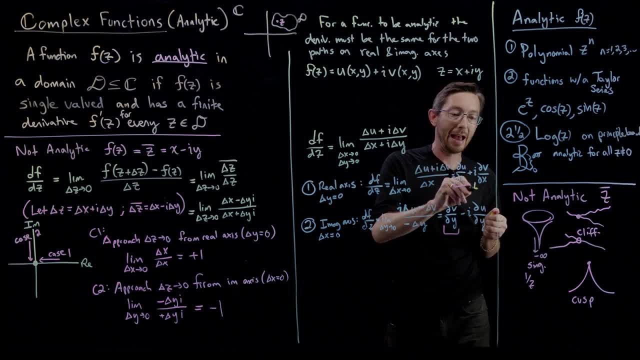 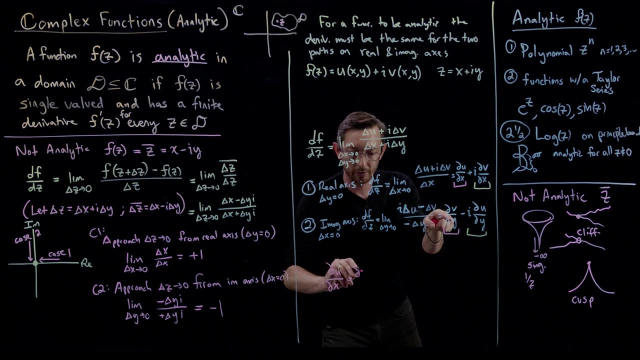 those have to be equal and also the imaginary parts also have to be equal, and these are going to give me my two Cauchy-Riemann conditions. so for my function to be analytic, i need partial u, partial x to equal, partial v, partial y. that definitely has to be true. and i need 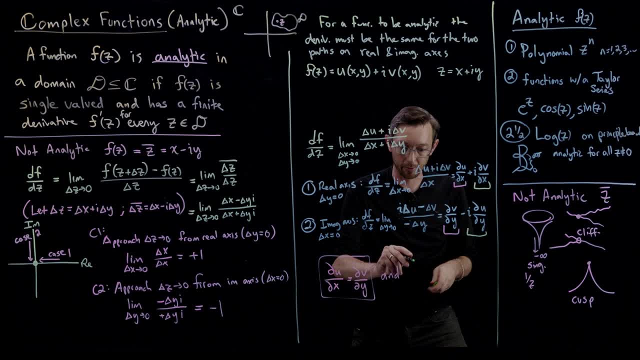 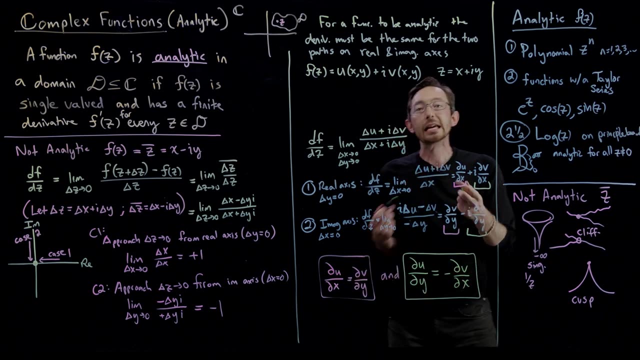 partial v, partial x, or let's say, you know, partial, uh, yeah, partial partial u, partial y to equal minus partial v, partial x. these are my two Cauchy-Riemann conditions, super duper important uh, Cauchy. some people think it's couchy, it's Cauchy and Riemann. 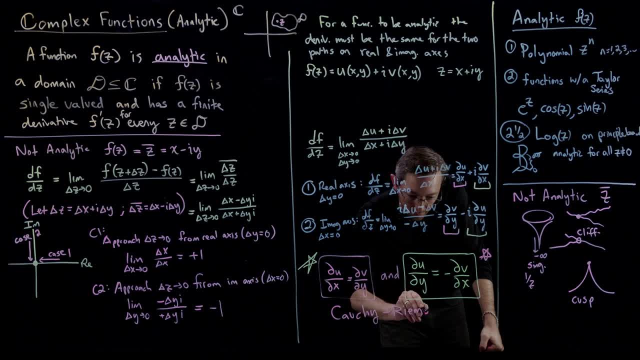 and how many m's and r's does Riemann have? Riemann, let's say, it's Riemann. i think there's probably two m's. i'll just put another one there, Riemann. okay, the Cauchy-Riemann conditions. so Riemann was Gauss's student, i think. 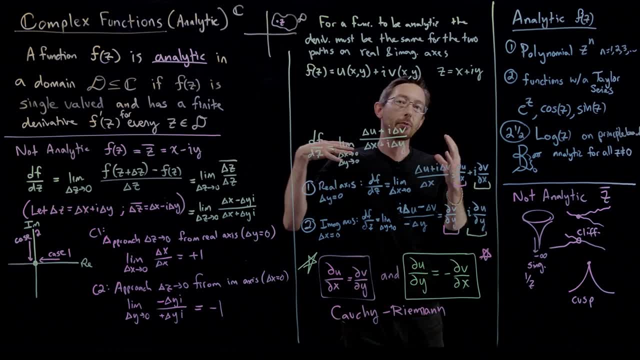 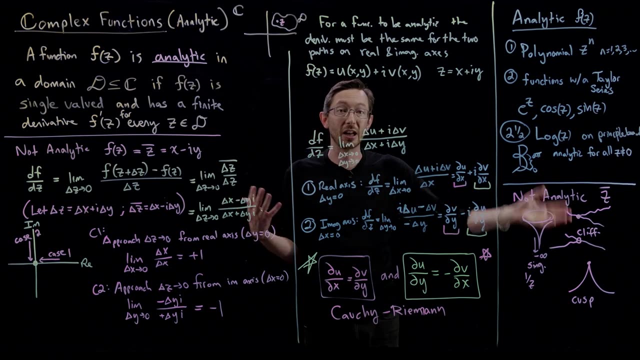 very, very, very bright geometer. Cauchy was probably one of the most influential people in making complex numbers real and concrete for us humans, along with Euler. so remember, before Cauchy and before Euler, people thought that imaginary numbers were just some useful computational trick, but they didn't really mean anything. they weren't real and Cauchy helped to solidify that. 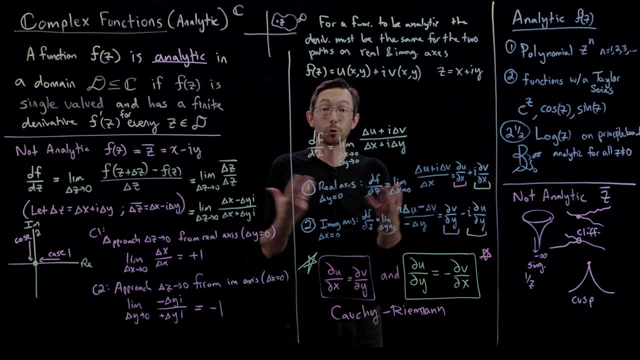 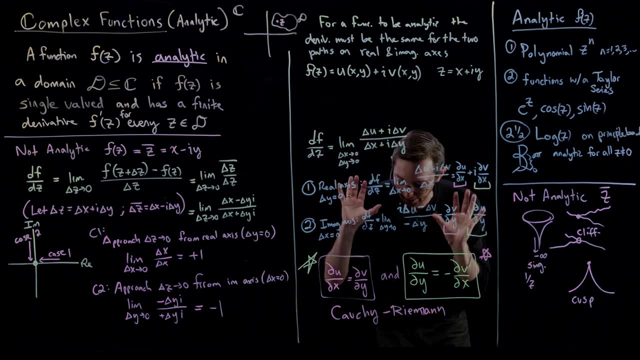 complex numbers and complex functions are actually, you know, essential parts of reality. they are solutions of physics, they are real, you know, concrete objects- and this is one of the most important uh conditions in all of mathematics- are called the Cauchy-Riemann conditions. if the real 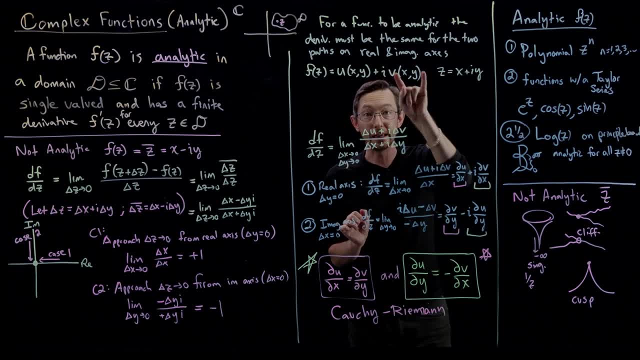 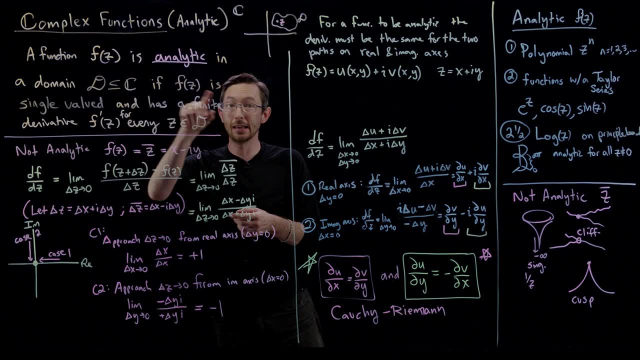 part u of my function and the imaginary part u of my function and the imaginary part u of my function satisfy these two conditions. what that means is that my derivative exists and will be finite, regardless of what approach i take. this delta z goes to zero if i go in the real axis. 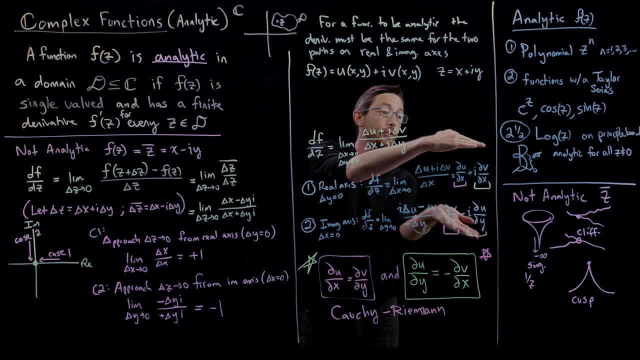 or the imaginary axis. if these two conditions are true, then these two expressions will be equal and, and my df dz is well defined, without having to specify what direction i took that derivative in. so this is a huge deal, okay, huge, huge deal. the Cauchy-Riemann conditions are necessary and sufficient. well, they're necessary. 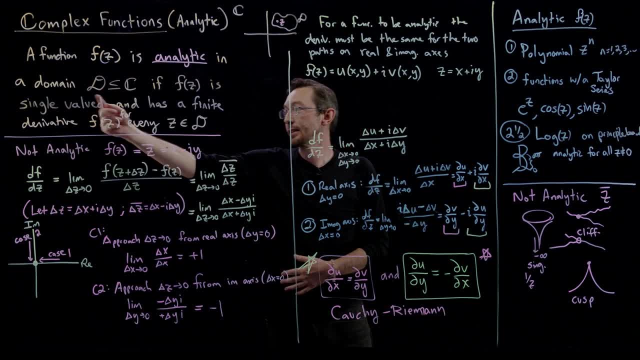 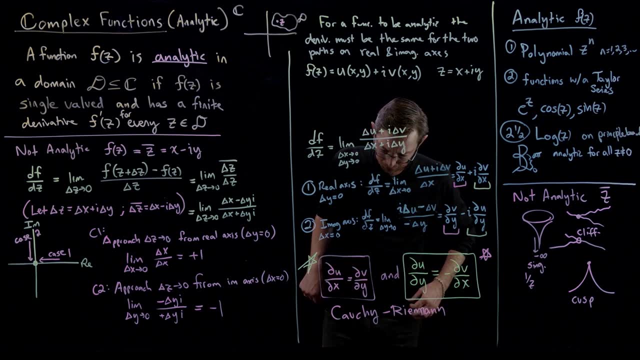 conditions for a function to be analytic. and if my function is single valued, um, you know, and these partials exist, then they're also sufficient conditions, very, very important, okay, so where is this going um? so that that's kind of it. we, um, you know, we're talking about complex functions. 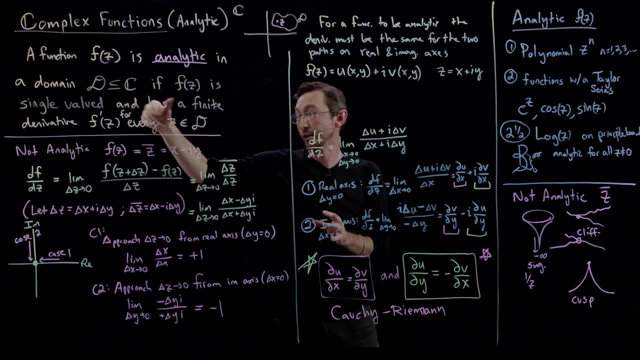 uh, that we can do calculus on. they're called analytic and they have these properties. basically, f prime of z exists. it's very easy to take data about these conditions, as well defined, regardless of what direction i take, that derivative in these Cauchy-Riemann conditions have to be true for my 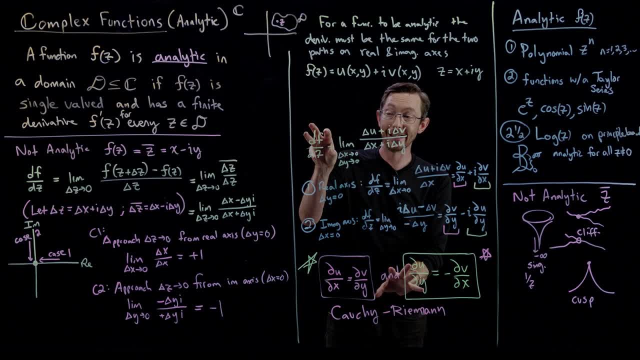 derivative to be independent of the path i take dz to zero on, and that is necessary and sufficient to have a well-defined derivative so that i can do calculus, functions like polynomials, exponentials, cosines and signs, and even the logarithm on its principal branch away from 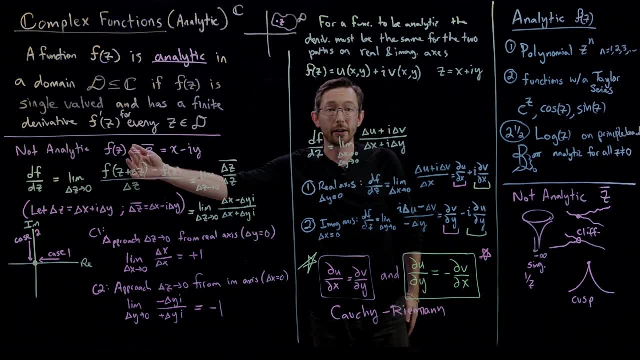 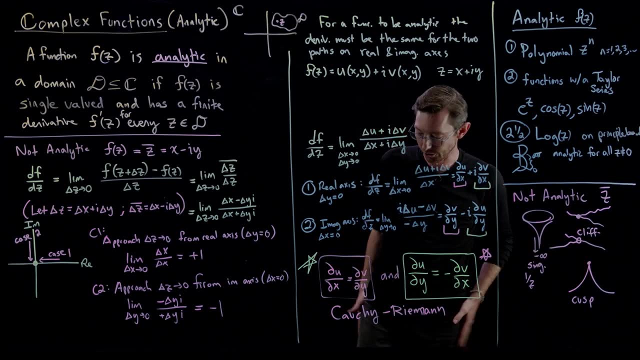 the origin are examples of analytic functions like the complex, conjugate or singular. you know, points at a singularity, or cliffs or cusps are typically not analytic functions. And why do we care about these analytic functions? What do they allow us to do? So analytic functions are super neat, because analytic functions essentially what? 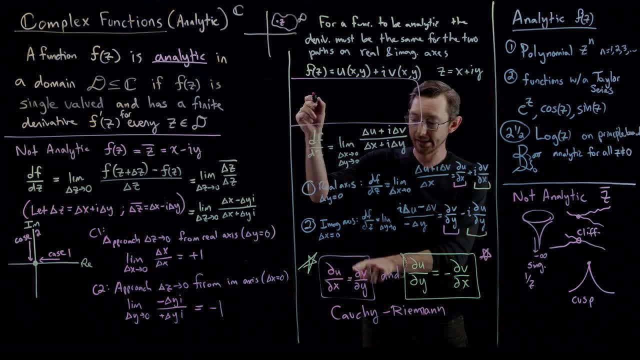 I'm going to show in the next lecture- very, very important lecture- is that if the function is analytic, if f of z is analytic, then the real part and the imaginary part solve Laplace's equation. Then del squared u equals zero and del squared v equals zero. So these analytic functions, 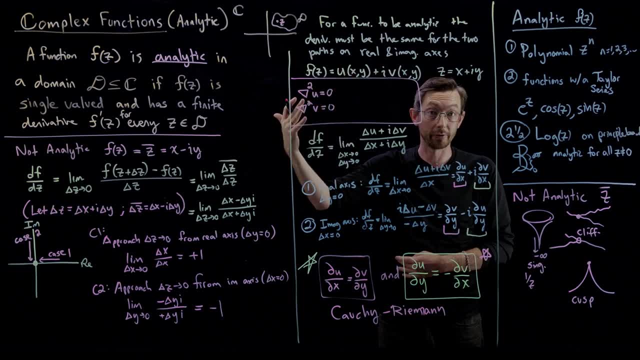 the real and the imaginary part solve the Laplace partial differential equation. These are called harmonic functions. The real and imaginary part of an analytic function are called harmonic functions. These are harmonic. And they're harmonic because they're the solutions, you know, of guitar string waves and sound waves. 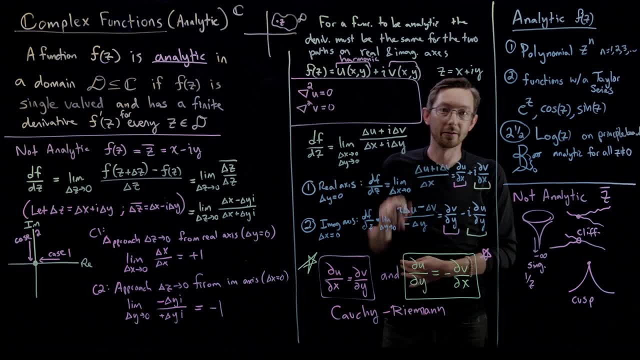 and all of the physics that you're used to. you know that involve kind of partial differential equations. The basis functions that we use to represent all solutions of, you know, simple linear PDs that we're familiar with are these harmonic functions like sines and cosines and 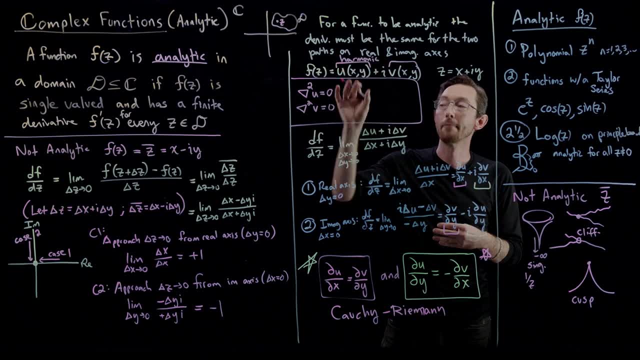 things like that. The Fourier series are harmonic functions that are the real and the imaginary part of complex valued analytic functions that happen to solve Laplace's equation. So if you're used to solve Laplace's equation, So that's super duper important, And before computers this is important. 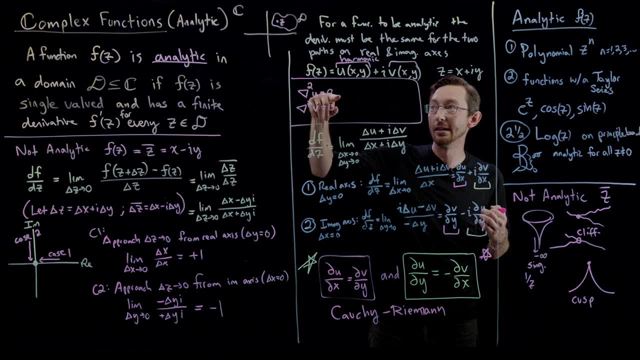 before computers, we had to solve these PDEs using by hand solutions pulled from the real and the imaginary part of complex functions. So, if you go back in time 50 years, complex analysis was not a two-week boot camp on YouTube, It was a full semester course that you took. It was a 15-week. 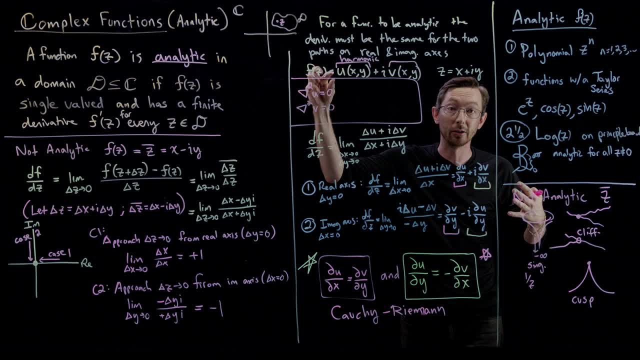 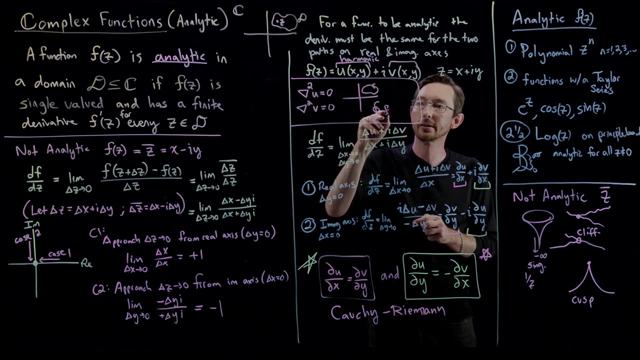 course, to get so good at dealing with these functions that you could actually solve really, really hairy, gnarly PDEs by hand. Okay, And then the last thing I'll show you is that if a function is analytic, there are some really nice properties of you know, solving closed contour integrals of 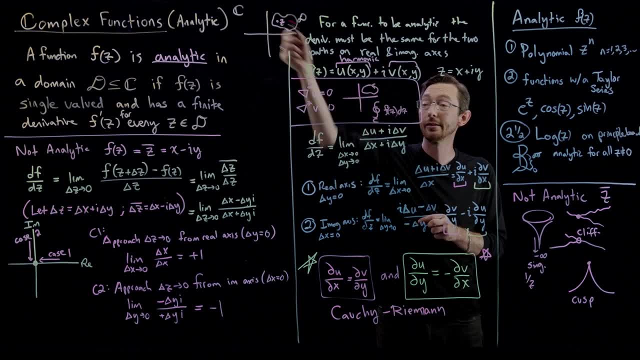 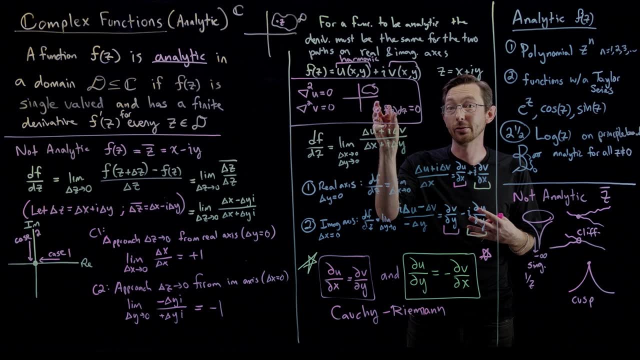 f of z dz over a closed contour that's inside this domain. that will equal zero. So that's a really, really important property of analytic functions is that it's really also easy to integrate them over closed loop, Just like we have conservative functions in physics. 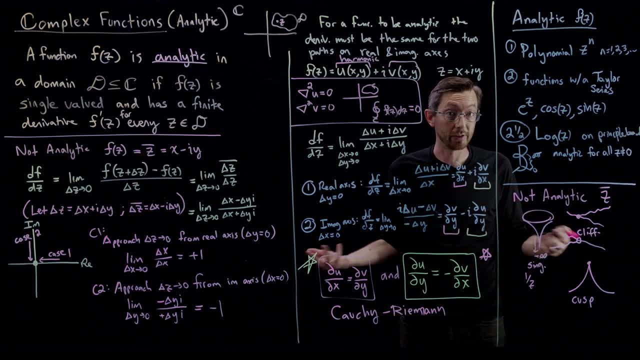 functions that conserve energy, like the potential function, the gravitational potential or the electrostatic potential, hint solutions of Laplace's equation. If I, you know, if I take a frictionless roller coaster and I go around that roller coaster and I end up where I started, 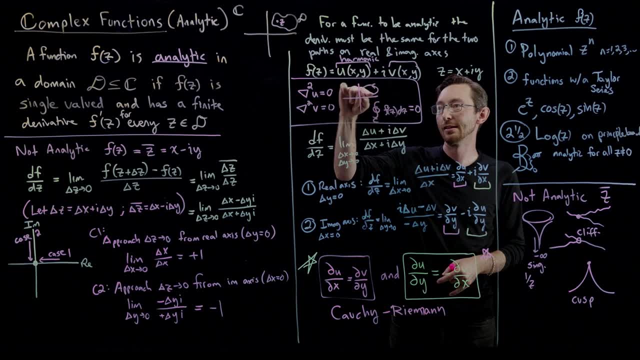 I have neither gained nor lost any energy, And that's kind of this generalization that all of these closed contour integrals inside of an analytic domain, of an analytic function, will add up to zero. They're kind of conservative functions. Okay, That was a huge amount. You'll probably have to, you know, go through parts of this again. 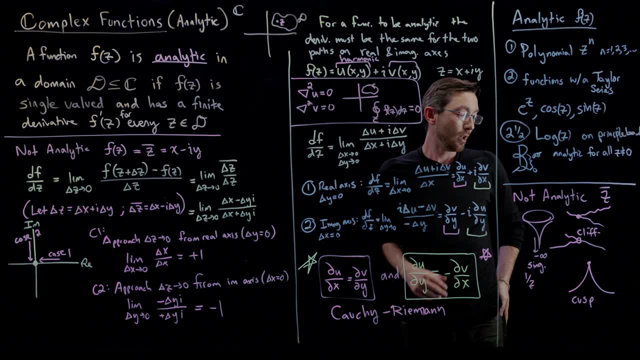 if you really want to master this. this is not trivial stuff. If you want, I'm going to probably erase this in fast forward and show you that z squared is in fact analytic. But this is kind of the end of the video, So in the next video I'm going to show you that, if my function is analytic, 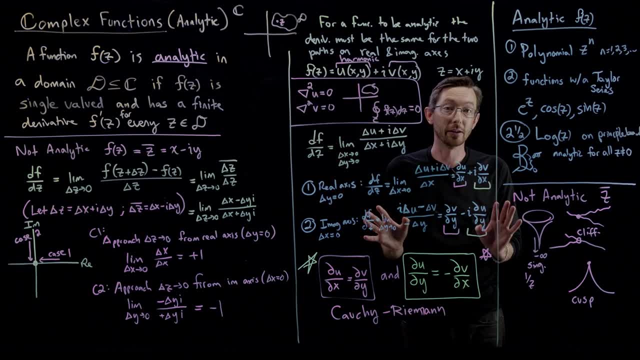 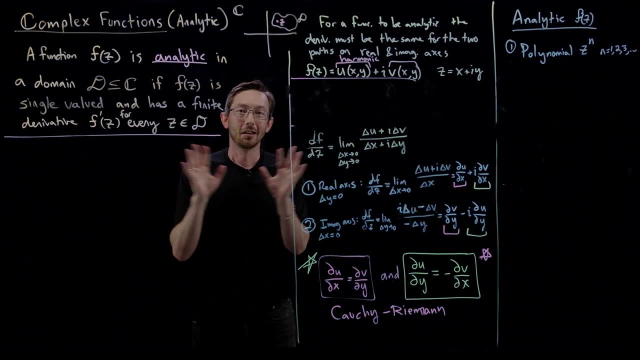 it does solve Laplace's equation Very, very important. All right, Thank you. Okay. So right now I'm going to show you that the polynomial z squared is analytic because it is single valued and because its derivative f prime exists regardless of the 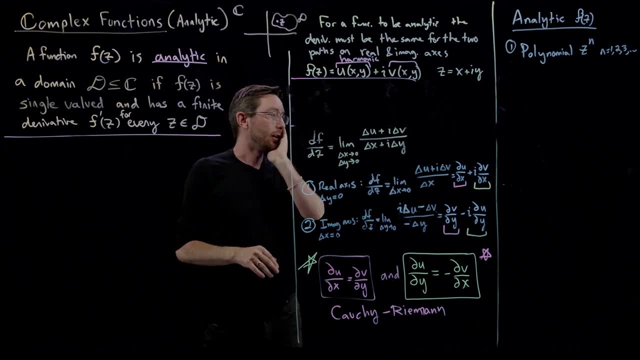 direction that I take. delta z goes to zero. Okay, I erased the board. I actually tried to do this and got myself completely stuck. These things are not always obvious or easy, So I get stuck all the time doing this kind of stuff. Maybe I'll leave that part in and 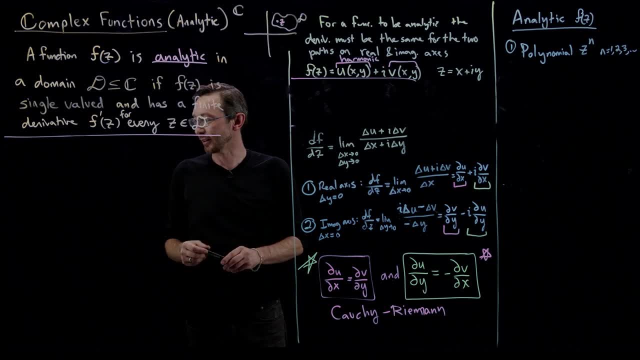 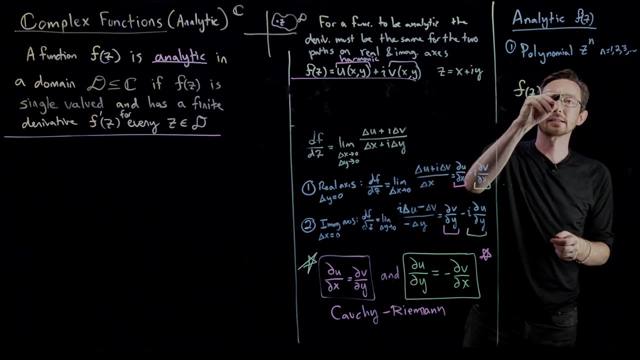 you will have just seen me fast forward through scratching my beard for about five minutes, But it's actually pretty simple. What I'm going to do is we're going to take the function f of z equals z squared. Again, this is a single valued function. If I pick a specific z, there's only. 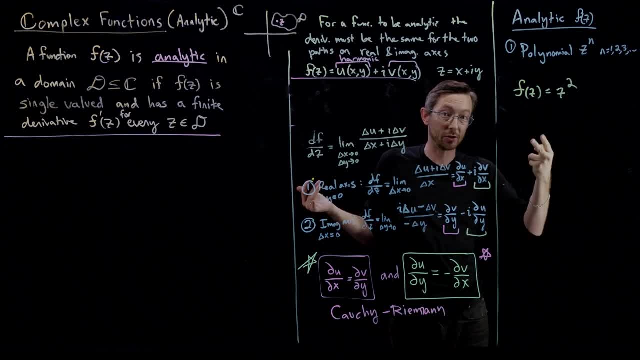 one number, z squared, unlike z to the one half, which has two values. z squared has one value, so it's single valued. And what we're basically going to do is we're going to take the function of f of z squared and we're going to take the function of f of z squared and we're going to take the. 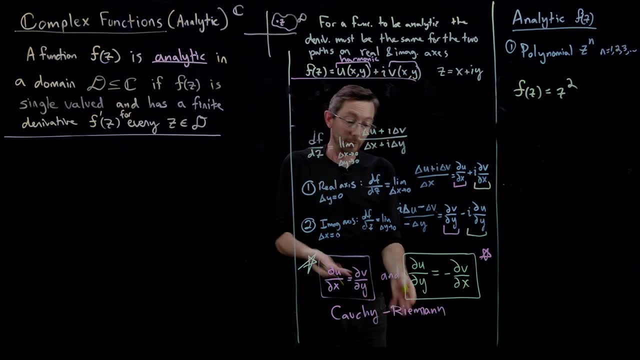 function of f of z squared. and we're basically going to do is, we're going to compute, We're basically going to show that the Cauchy-Riemann conditions hold, so that the derivative along the real axis and the derivative along the imaginary axis are equal to each other. Good, So f of z. 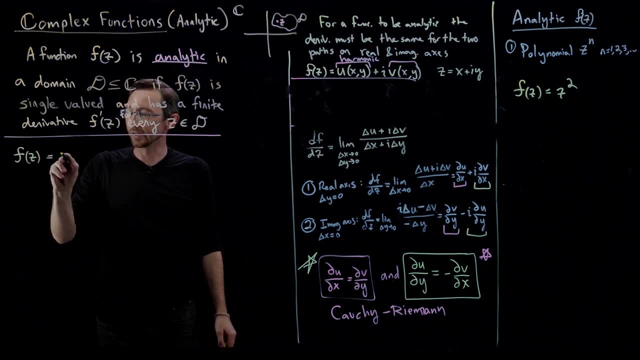 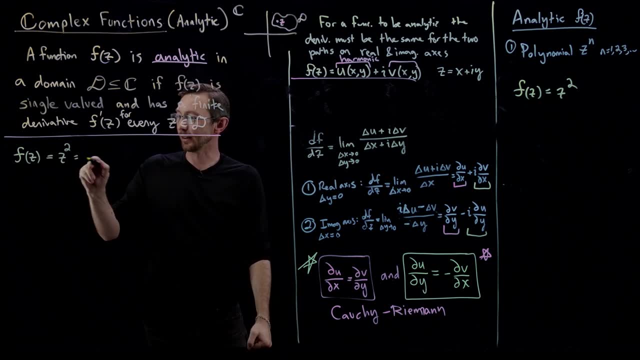 f of z equals z squared, And I'm going to write this out in the real part plus the imaginary part. So this equals, you know, it's like x plus i, y, quantity squared. So the real part is going to be an x squared, And I'm going to write this out in the real part plus the imaginary part. 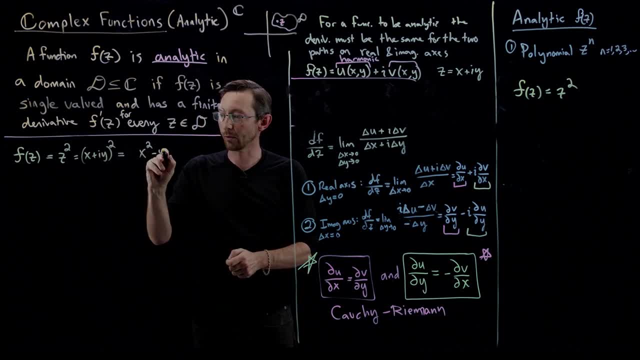 So this equals x squared plus an i, y quantity squared, which is minus y squared. That's the real part, Plus i times, you know, x y plus y x. So that's i times 2 x, y, And so this is my real. 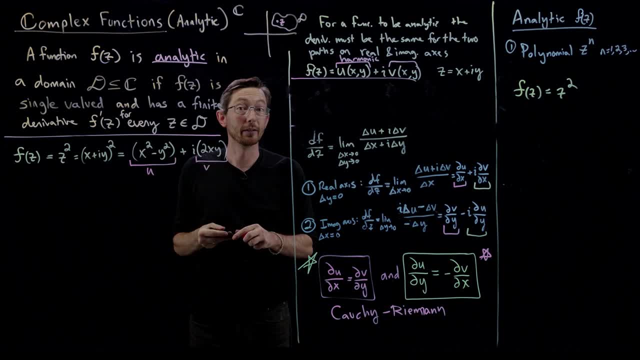 function u and this is my imaginary function v. Good, And I think what I'm going to do, because we know, you know, if we approach on the real axis, then the derivative, the derivative is equal to this sum of partials, And if we approach on the imaginary axis, 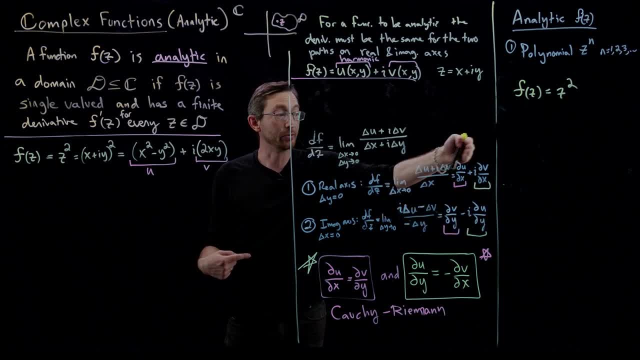 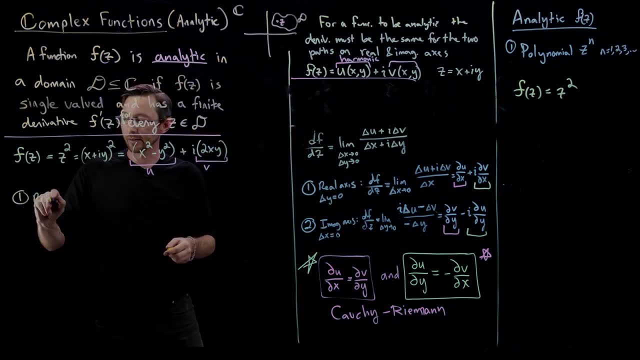 the derivative is equal to this sum of partials. I'm just going to compute these two partials and confirm that they're equal to each other. Okay, So along path one, if I go on the real axis, the real axis path of delta x goes to zero. then df, dz. 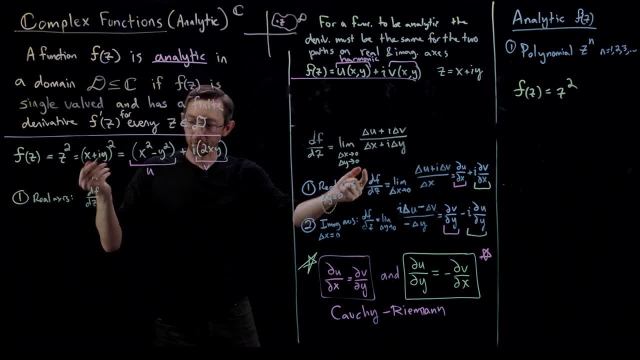 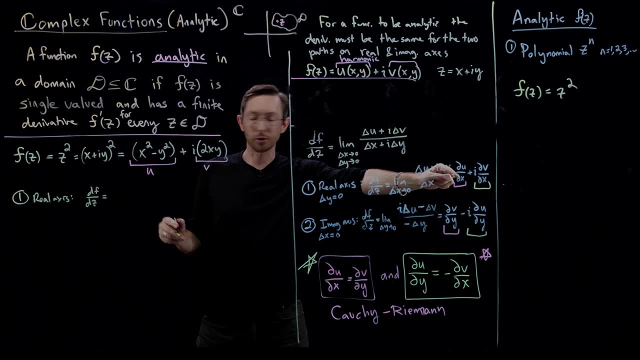 df, dz, which is essentially df. you know the limit of delta f over delta x. This is going to equal partial u. So I'm going to write this out in the real part plus the imaginary part, plus the partial u: partial x, partial u, partial x plus i, partial v, partial y And partial u. 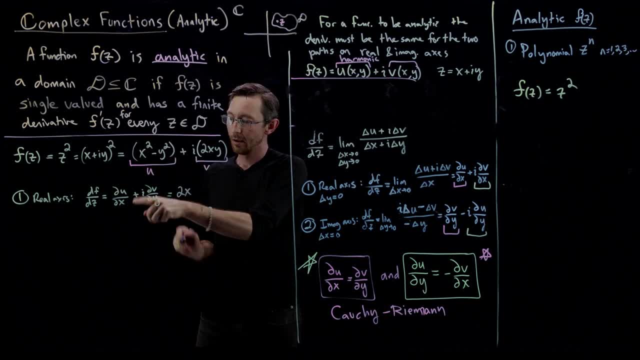 partial x is 2 x plus i, And partial v, partial y is again 2 x, correct 2 x. Did I do that right? Oh well, I'm stupid. This is partial v, partial x. Sorry, I'm not stupid. No one like when you. 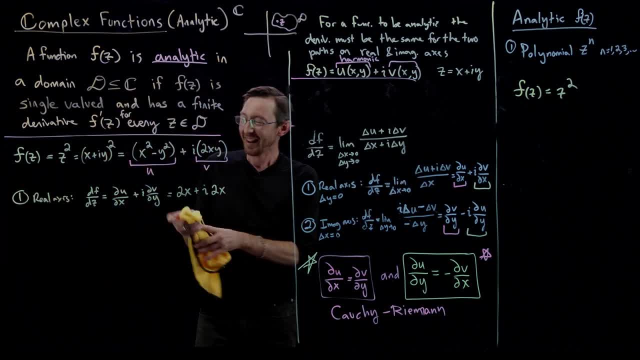 make a mistake. you're not stupid. It was a stupid mistake. This is not partial v, partial y. here It's an obvious mistake. Dumb mistakes are the best mistakes because they're easily fixed. Okay, That's what I always tell my students when they, you know, finally found a bug in their code and 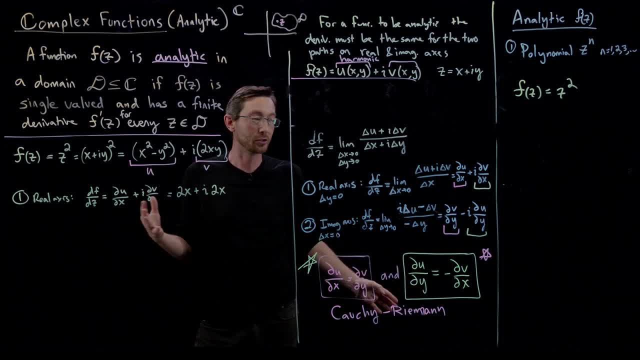 they feel, you know, like it was the simplest mistake and they've been stuck on it for two weeks. Those are the best kinds of mistakes because they're so easy to fix. Okay, So dumb mistakes are the best mistakes. This wasn't partial v, partial y, It's partial v, partial x. 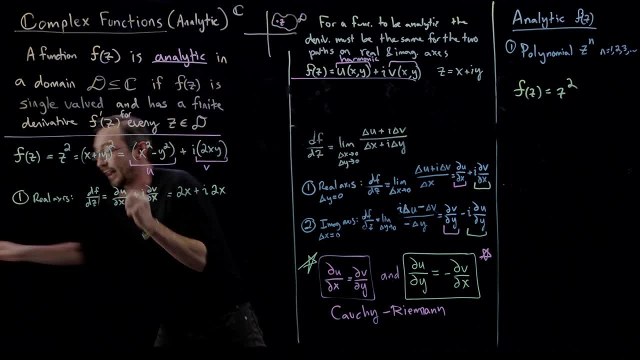 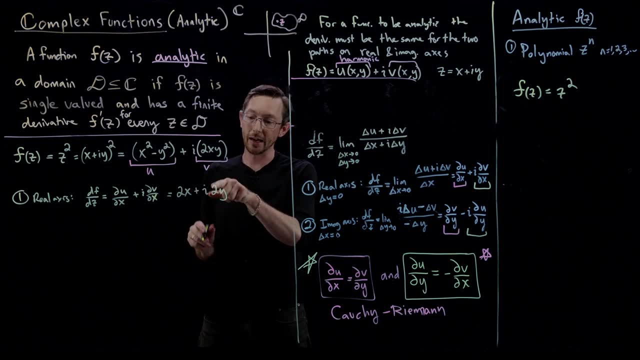 And partial v, partial x. if I take the derivative, I get a 2 y. That is more like what I'm looking for. This becomes a 2 y And 2 x plus i. 2 y equals 2 x plus i y, which is 2 z. Beautiful, Okay. 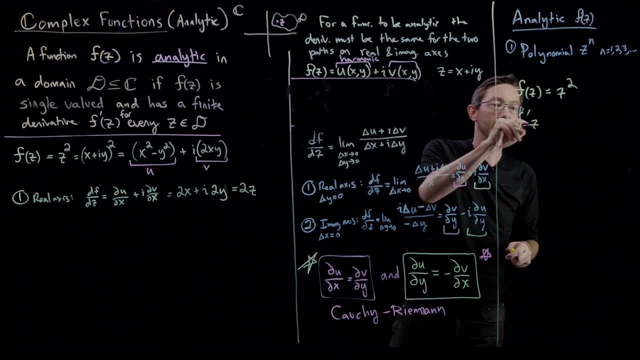 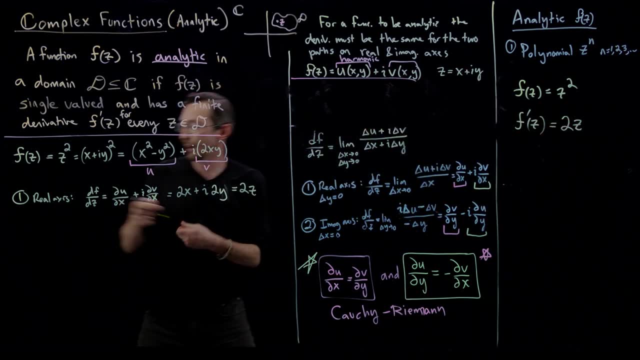 That's what I expect my derivative to be. I expect my derivative f prime of z intuitively to be 2 z. That's what we expect from regular calculus. So that's true when I do this way. Now let's try it. 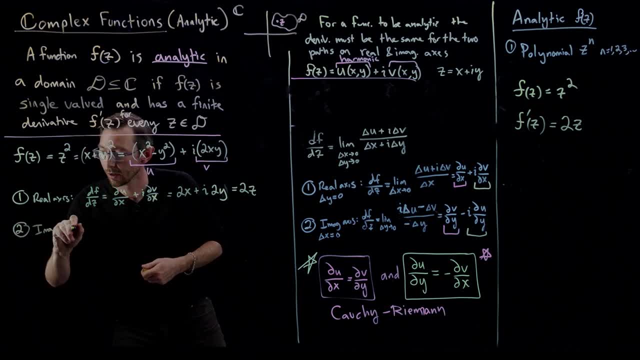 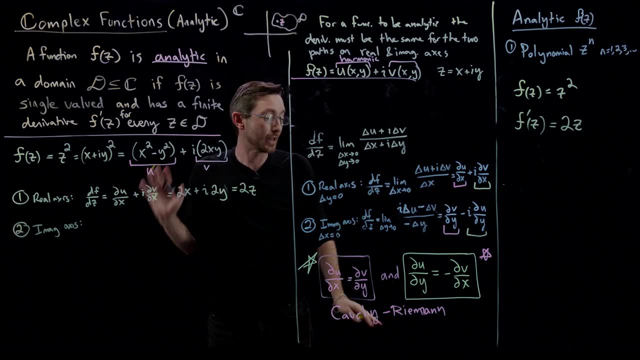 on the imaginary axis, Image axis, Okay, And I think it's important for you to see me make mistakes, because I mean I make mistakes all the time When I do this live for my students. sometimes I actually prepare only a certain amount so that they can see you know how you derive things on. 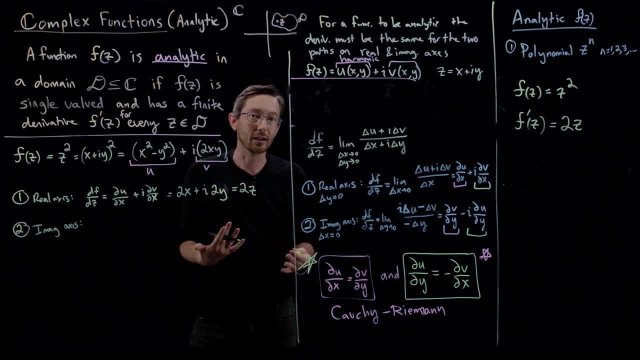 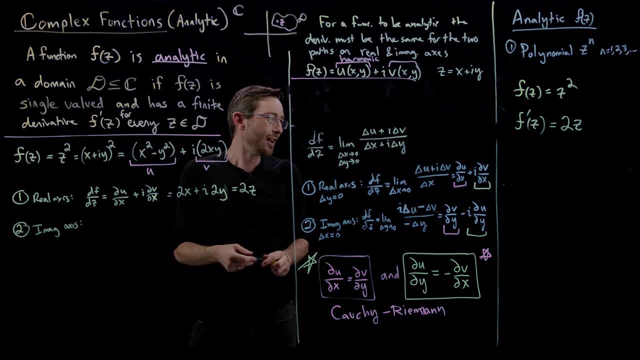 And they remember everything and they always can solve the answer. I mean, that's probably not the case. Okay, We all make mistakes and we all have to be catching ourselves constantly. So now, if we compute this on the imaginary axis, we have df. dz equals- this is just a straight line. d- This is a. 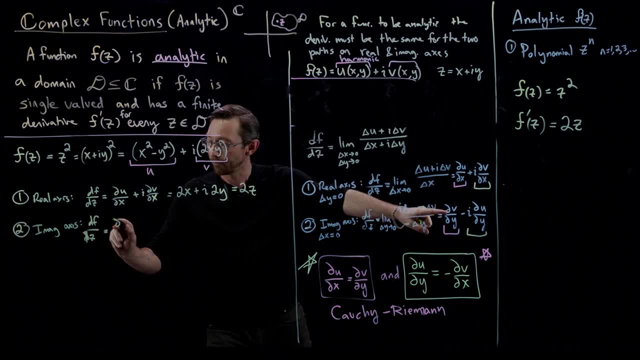 total derivative df dz. It equals partial v, partial y minus i partial u, partial y. Okay, Good. Partial v partial y is 2x. Good, Minus i. partial u partial y is a minus 2y, So that's a. 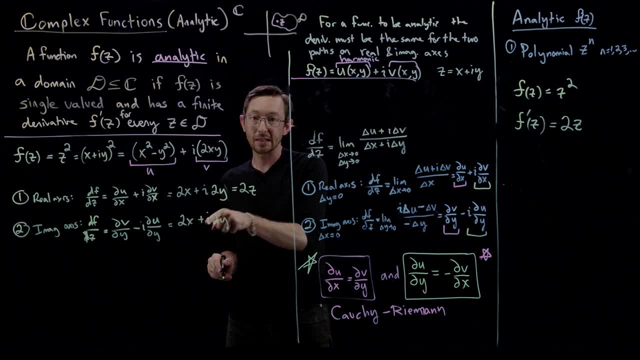 minus 2y And again 2x plus i. 2y is just 2z. So essentially, what this shows is that, because these two equal each other, this derivative, this function f of z equals z squared. the derivative. 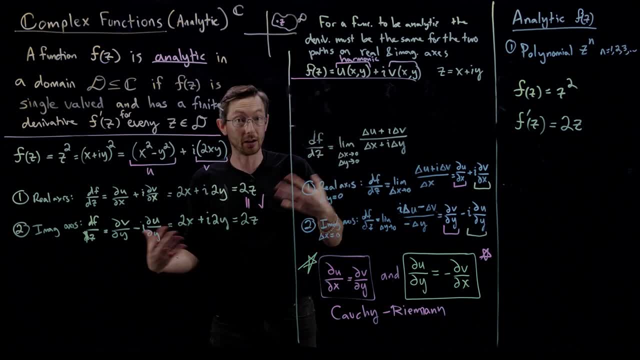 is 2z, Regardless of what direction I take it in the complex plane. Now, if you want to get really, you know good at this and you have 30 minutes to do this on your own, I would recommend you know. 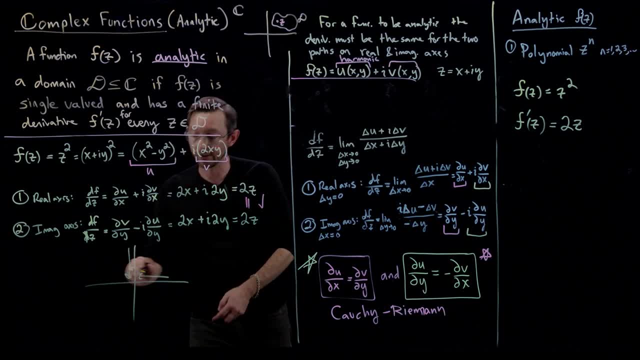 we just took the derivative in the real direction. We just took the derivative in the imaginary direction. Confirm for yourself that if you take the derivative in, you know this direction of like delta x equals delta y goes to zero, or in this direction, those also equal 2z. It's a little. 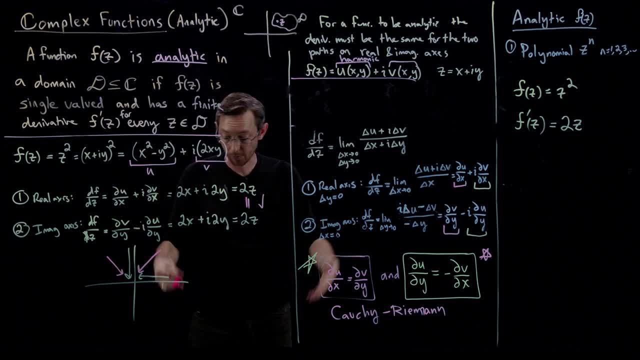 bit hairy. You're going to have to figure out how to do that. But if you take the derivative in the real direction, you're probably going to have to Taylor series, expand this thing and keep track of a bunch more stuff. But it definitely is true And that's kind of how you would prove that this Cauchy-Riemann condition. 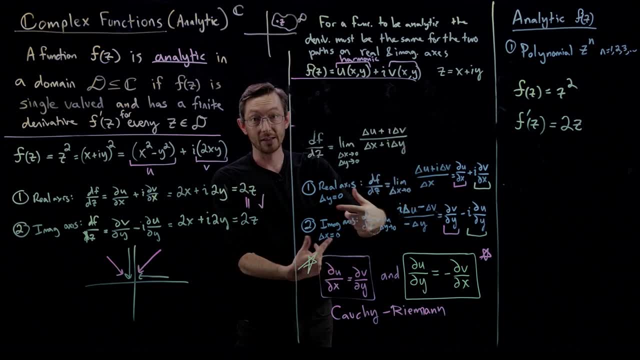 you know that the real and the imaginary direction derivatives equal each other, is necessary and sufficient that the directions will. you know that the derivative is well defined. for any direction, delta x and delta y go to zero. For any path I take, where delta x and 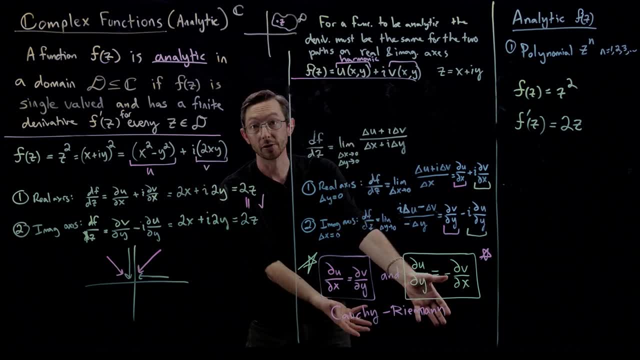 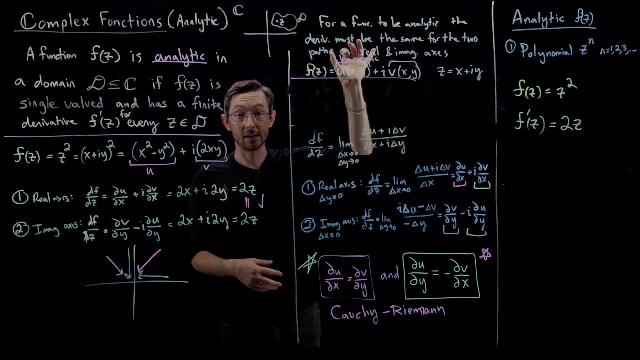 delta y go to zero, they're all going to equal each other if these two conditions are true. Okay, so next lecture, we're going to prove that the real and imaginary parts of these analytic functions are solutions of Laplace's equation called harmonic functions, And we're 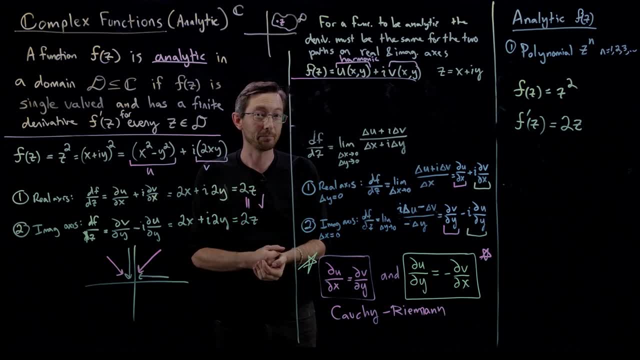 going to derive some kind of important consequences of that. All right, stay tuned, Thank you.